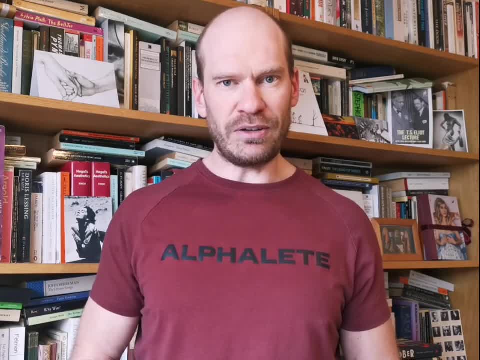 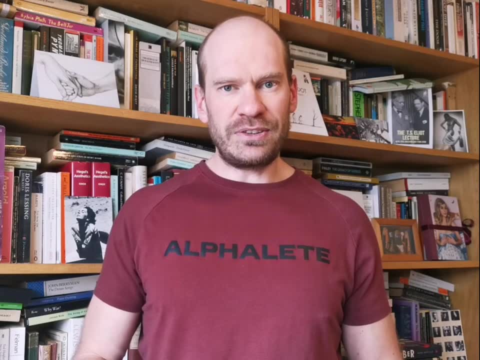 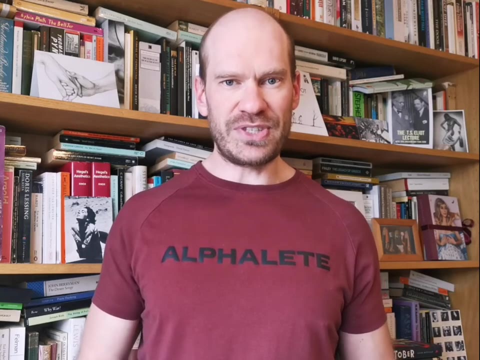 or the frequency domain, and also in terms of a complex variable, z. We will see the physical interpretations of these Green's functions and how to actually just go ahead and calculate them for a given simple system. The system we'll start with is the simplest possible system of a time-independent single. 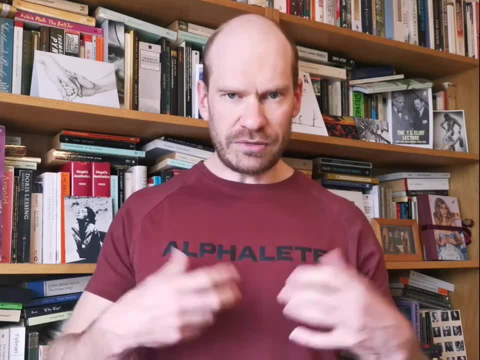 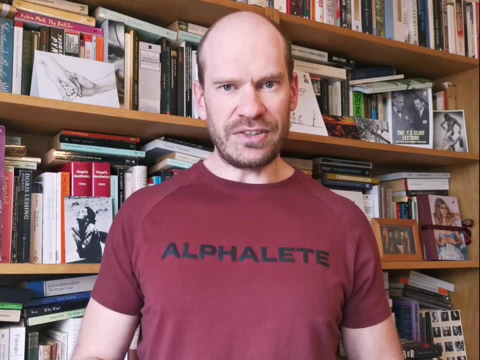 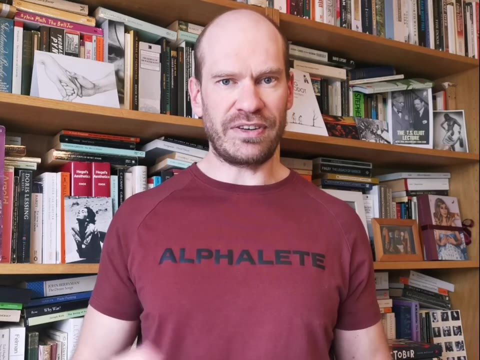 quantum orbital with a particular level energy and we'll derive all of the Green's functions for this system. We'll talk about how the retarded Green's functions are related to the density of states of the system. We'll also talk about the fluctuation-dissipation theorem and how the Green's 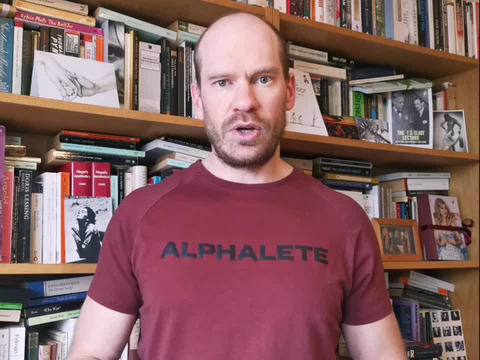 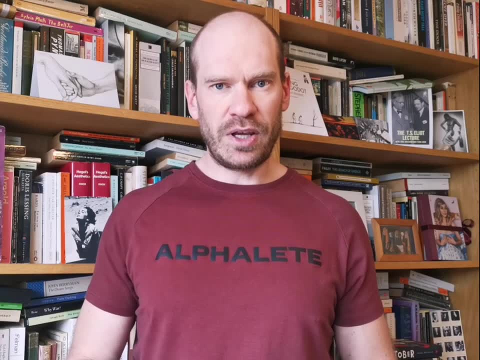 functions are related to orbitals. We'll also talk about the flux-dissipation theorem and how the Green's functions are related to orbitals. We'll then have a look at a time-dependent Hamiltonian and we'll go through the same process again for this non-equilibrium situation. We'll look at the situation of a so-called quantum. 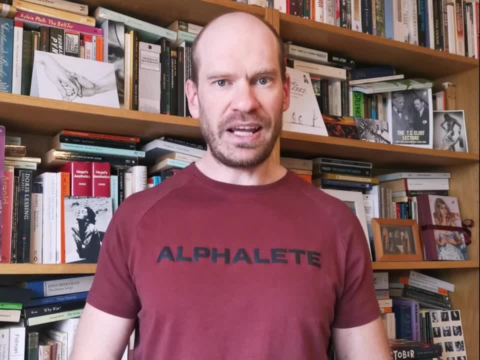 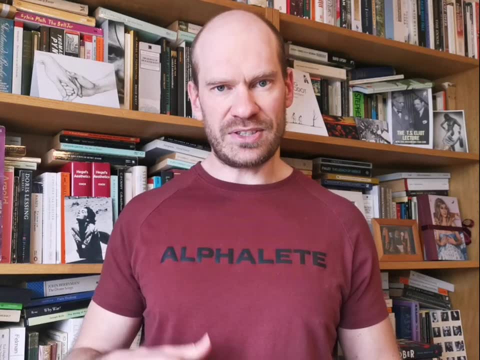 quench, where we suddenly change the Hamiltonian at t equals zero and see how the dynamics of the system evolves. Finally, we'll have an outlook towards systems with many quantum orbitals, which is of course what we want to look at in this course. In the coming lectures we'll return to this and we'll be developing first the Green's functions. 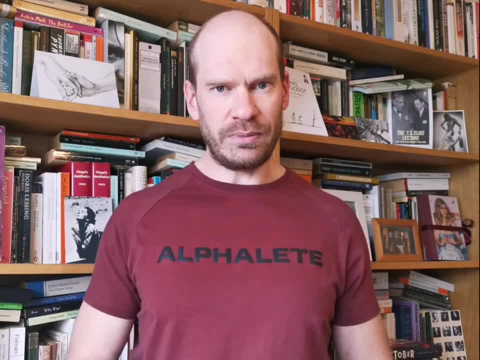 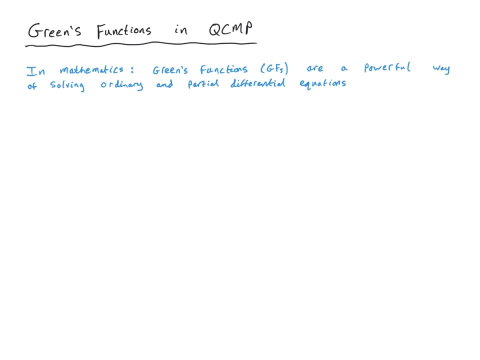 But the foundational material will be contained in this lecture. So let's get down to work. In this lecture we'll be discussing Green's functions in the context of quantum condensed matter physics. But before we get into that, let me give some of the mathematical background. 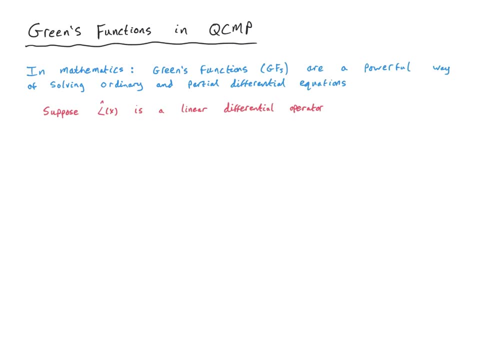 behind the theory of Green's functions. Suppose that we have a linear differential operator, L hat, which is a function of the coordinate x. Let's say that we then wish to solve differential equations of the type: L hat, acting on u of x is equal to f of x. So here we have on the right-hand, 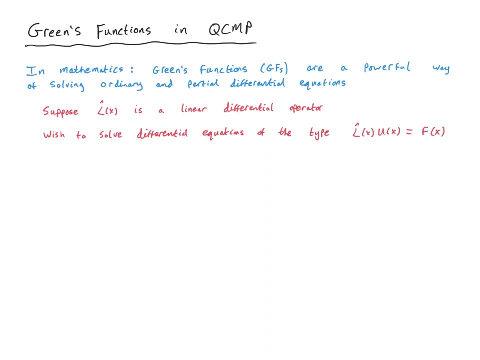 side a source term f of x and the linear differential operator L hat on the left-hand side, and we want to solve this equation for this function, u of x, Which u of x, when operated on by L hat, gives us the source term f of x. One way of solving differential equations of this type is: 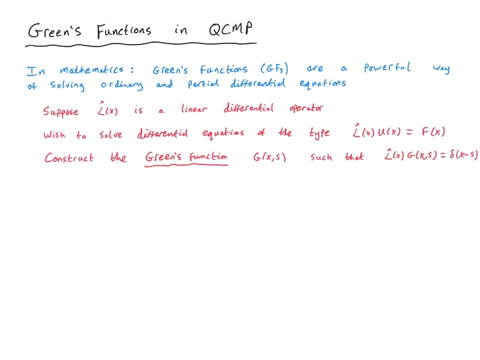 to use Green's functions. We construct a Green's function g, which is a function of x and s, such that when L hat acts upon the Green's function, we get the delta function, the Dirac delta function, delta of x minus s, By multiplying both sides of this equation by f of s and then integrating over s. 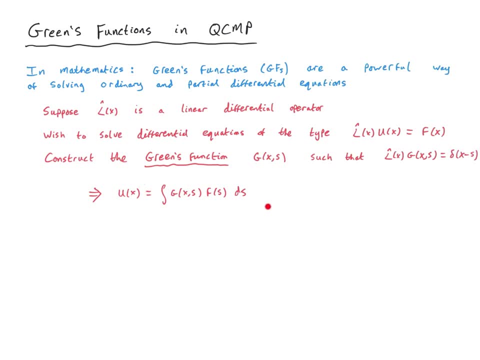 we then easily obtain a solution to u of x. So if we know the Green's function g of x and s, we can easily find solutions to differential equations of this type. Some of you may have already encountered Green's functions in the context of classical physics. In particular, it's widely used in the theory of electrodynamics. 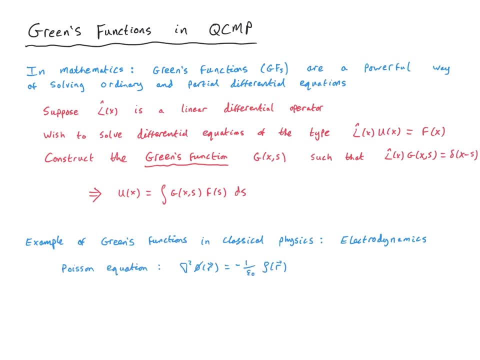 For example, let's take the Poisson equation where we have a differential operator which is the Laplacian del squared acting upon our electrostatic potential phi of r, and this is equal on the right hand side to minus one upon epsilon naught times u of x. So we have a differential operator which is: 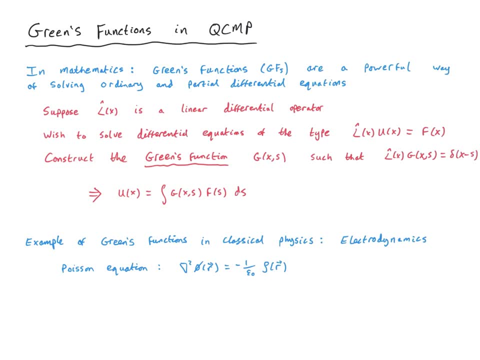 the charge density rho of r. In analogy to the above expression involving our L x operator, our solution u of x and our source term f of x. here we see that the differential operator L hat is the Laplacian del squared. the source term here is basically the charge density rho of r. 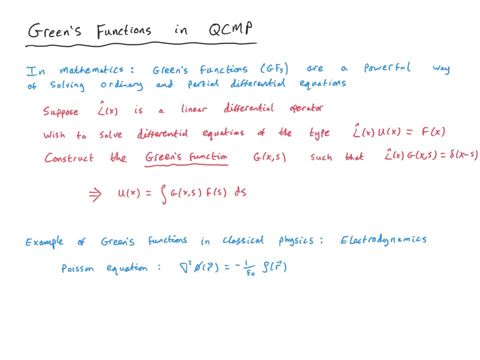 and the solution that we're after is the electrostatic potential phi of r. We can now introduce a Green's function g of x and s which is equal to the charge density rho of r In a translationally invariant system. however, we can express this in terms of a single variable. 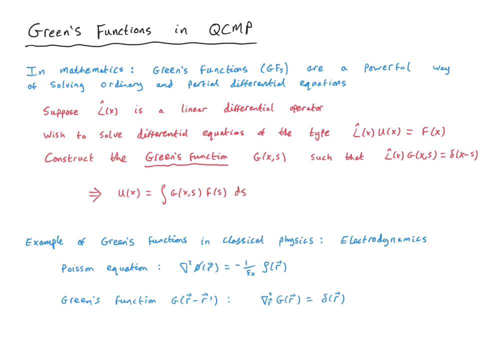 r minus r primed, We define our Green's function g of r such that, when we operate on it with our Laplacian, we get the delta distribution delta of r. Substituting this into the Poisson equation, we then find an expression for our electrical potential. The reason why this construction is. 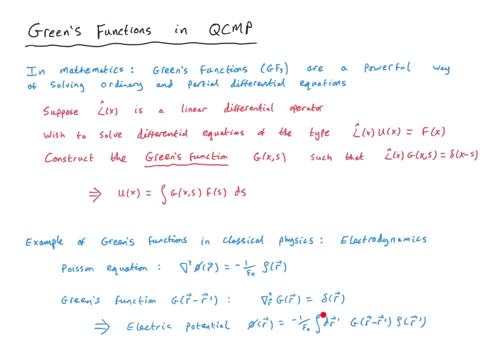 is that the defining equation for the Green's function here that Laplacian, acting on the Green's function, gives the delta function is a much easier equation to solve than the generic Poisson equation where the right hand side has some complicated source term In particular. we can solve the Green's function equation here in this case by means of a simple. 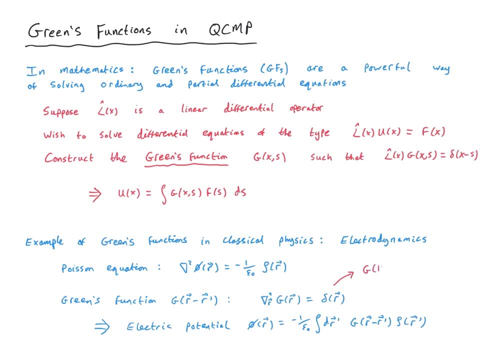 Fourier transformation: If we go to k space, then we find very straightforwardly that g of k is equal to minus one upon k squared, and I'll leave that as an exercise for you. Going back to real space, we can then substitute our expression for g of r into the equation for: 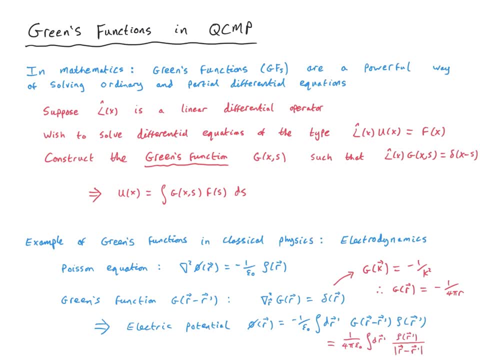 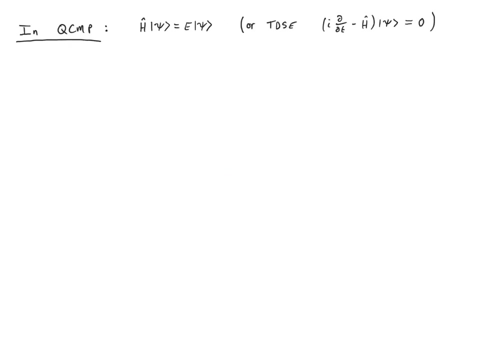 the electrical potential. This then immediately gives us the well-known expression for the potential created by an arbitrary charge: distribution. Okay, so how can we use this Green's function theory in the context of quantum condensed matter physics? Of course, in quantum condensed matter physics, the differential between g of r and g of r is very simple. The difference 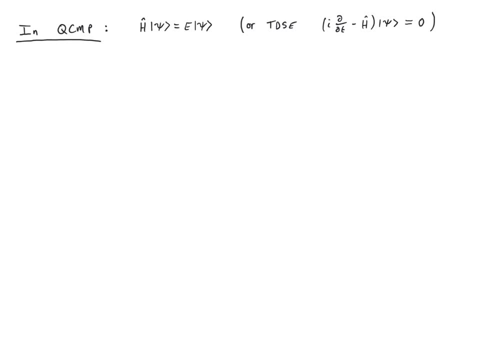 between the two is that the differential equation that we're interested in solving is the Schrodinger equation: h psi is equal to e psi, or likewise, the time-dependent Schrodinger equation i d by dt of psi is equal to h psi For a single particle Hamiltonian. we can then simply define: 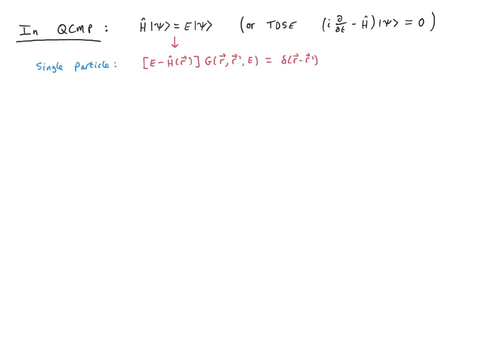 a corresponding Green's function which solves the Schrodinger equation. We can write that e minus h, acting on the Green's function, is equal to the delta function. Here I've allowed the Green's function to have arguments r and r primed, but on the right hand side we see that this is equal to. 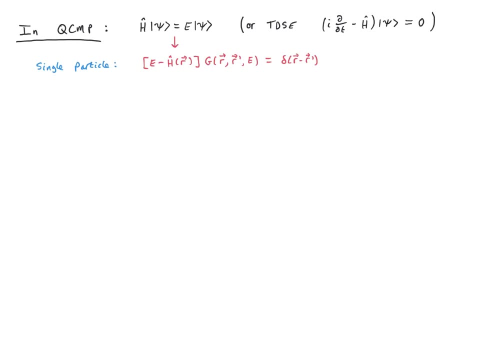 the delta function of r minus r primed. So in fact, r and r primed must enter in the Green's function only in the combination r minus r primed. In the position representation. the Green's function is therefore diagonal and we only have a single collective variable, r minus r primed. We can then 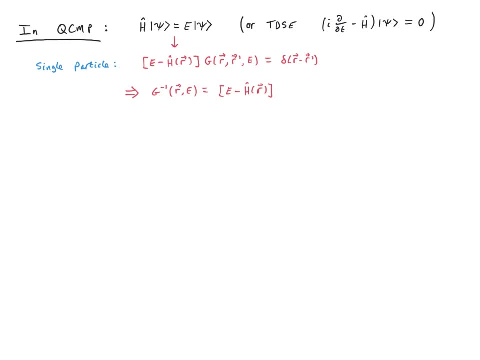 naturally identify the inverse Green's function, a variable r, as being simply e minus h of r. This then implies that g inverse of r multiplied by g of r minus r primed is equal to the delta function r minus r primed, as desired. This is nice because 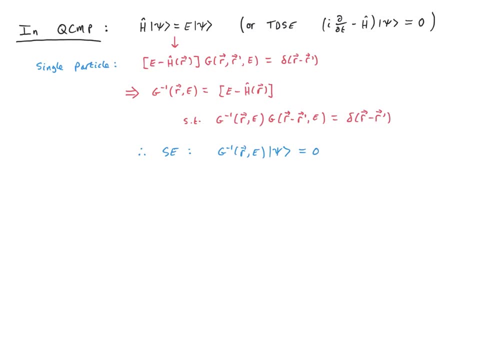 it provides an alternative way of writing the Schrodinger equation. g inverse acting on the wave function, psi is equal to zero. We can now play exactly the same game with the time-dependent Schrodinger equation which I've written again. here We introduce a Green's function g which now depends on the position r and the time t, as 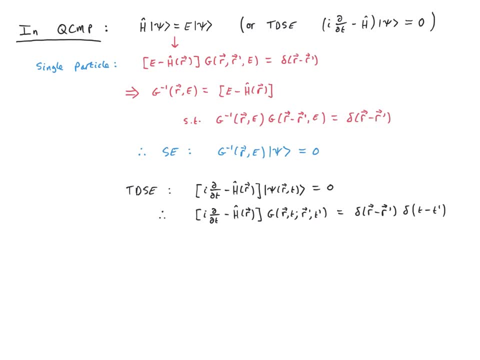 well as r primed and t primed. On the right hand side we therefore have Dirac delta distributions for position delta of r minus r primed, as well as time delta of t minus t primed. The same logic applies On the right hand side. we see that we have a function only of r minus r primed and t. 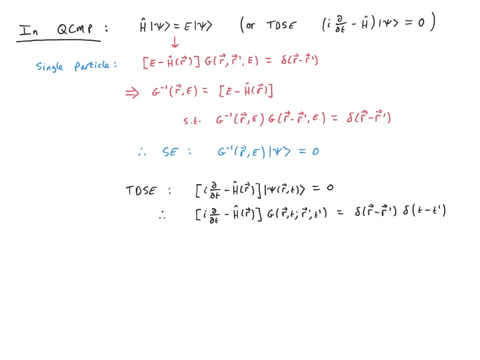 minus t primed. So we can define the e minus r prime of the length of the sine and the e of the inverse Green's function just as a function of those two collective variables. g inverse of r and t is therefore equal to i, d by dt minus h of r. From these equations it immediately follows: 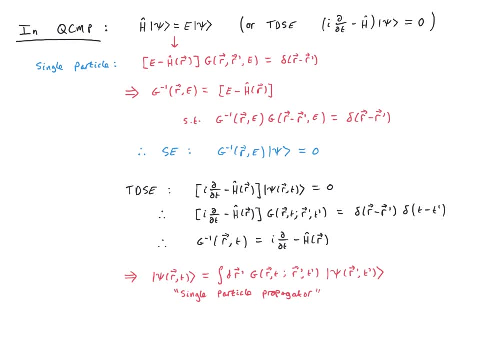 that the wave function psi of r and t can be expressed as the integral over all space of the Green's function multiplied by the wave function of r primed and t primed. This can be very simply verified by taking this expression for the wave function r and t and plugging it in the 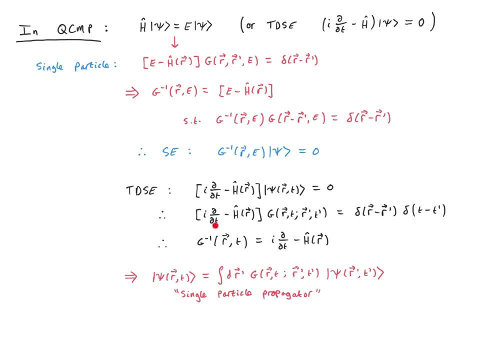 Schrodinger equation here, and then using the property that this object, in square brackets, multiplied by this Green's function, is equal to these delta functions. This expression therefore tells us that the Green's function can be understood as a single particle propagator. It relates the wave functions at time t, primed, to a wave function at time t and as. 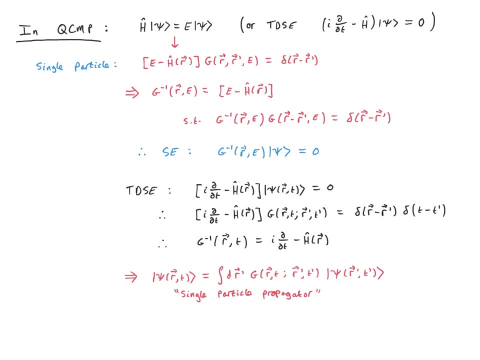 we can see here from the integral. this involves taking the particle at time t primed, at all possible positions r primed, and propagating it forwards in time to the specific position r. This is rather reminiscent of the Feynman path integral version of quantum mechanics, in which we imagine that the 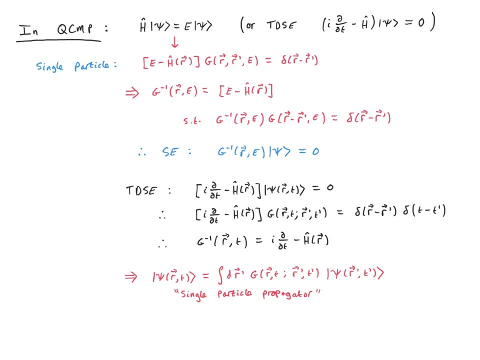 propagation of a particle from time t primed to t involves taking all possible roots from start point to the end point. In quantum mechanics, where the Green's functions refer to solutions of the Schrodinger equation, the Green's functions have a physical interpretation as the probability amplitude of taking a particle. 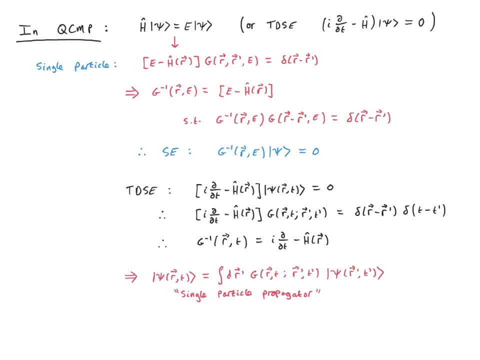 from position r, primed at time t, primed and ending up at position r at time t. If we now define the wave function at position r and at time t as the projection of the wave function psi of t onto the position vector r, And given that we know the solution to the time dependent Schrodinger equation for a single 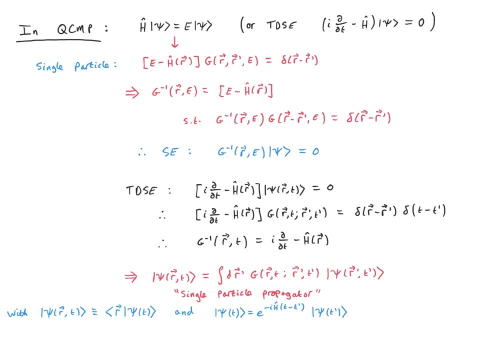 particle, which is written here psi of t primed, acted on by the time evolution operator e to the minus ih of t. minus t primed propagates the wave function forward to psi of t. then we can simply write the following, Where here I've simply taken this equation and now pre-multiplied by bra r and then interpreted: 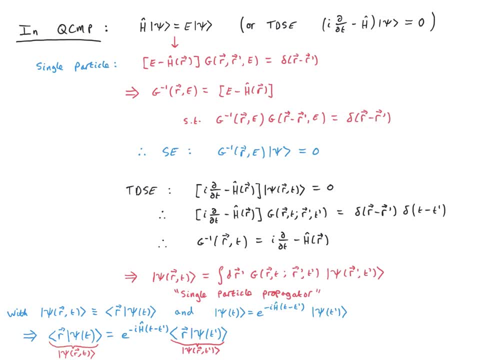 these brackets In terms of psi of r and t on the left hand side and psi of r and t primed on the right hand side. I can now insert a complete set of states inside this expression by simply multiplying by the identity operator: one hat. 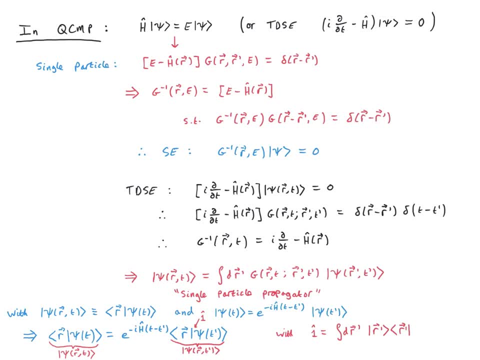 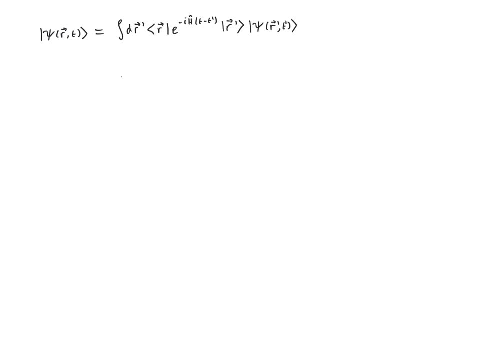 By resolving the identity operator as an integral over position, we then obtain the following: The wave function psi of r and t is therefore equal to an integral over dr, primed Of psi of r primed and t primed, multiplied by this matrix element that connects r to 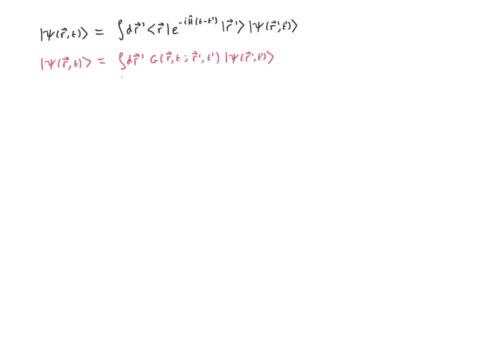 r primed under the time evolution operator, But using our Green's function formulation, we have a very similar kind of equation. Comparing these two allows us to get an explicit expression. in this case, for the Green's function, We can write that the Green's function g as a function r and t, and r primed and t primed. 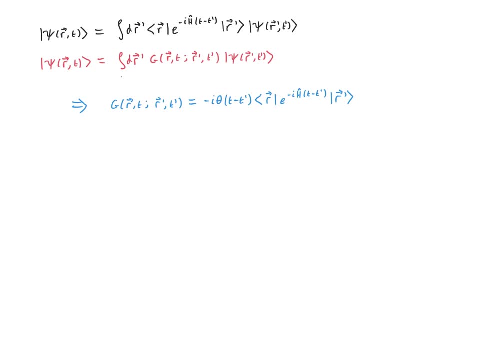 is equal to minus i theta of t minus t primed times. this matrix element, This theta function here, simply tells us that the time t must be greater than the time t primed. That is the order of the events, of the propagation that we defined in these equations. 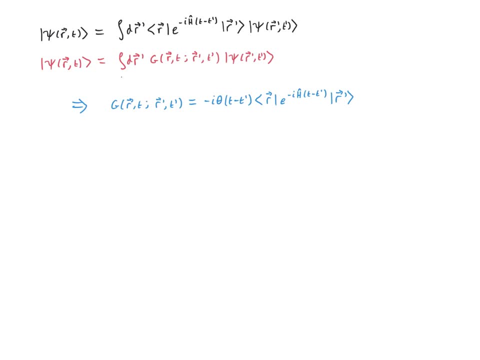 Theta of t minus t primed. here is simply the Heaviside step function. We start with a wave function at time t primed, and then we imagine propagating forward in time to psi of t. This defines the so-called retarded Green's function where t is greater than t primed. 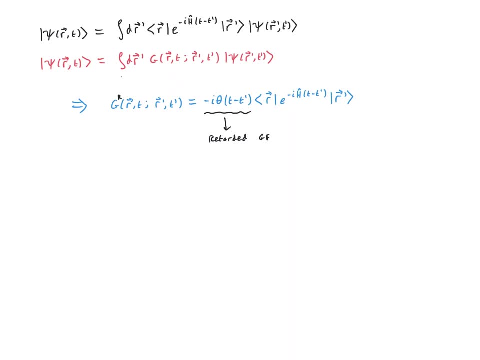 Sometimes you will see this denoted with the superscript r in the Green's function to emphasize that this is the retarded Green's function. A different but somewhat equivalent solution to the differential equations are the so-called advanced Green's functions, where here we have plus i, theta of t, primed minus t. 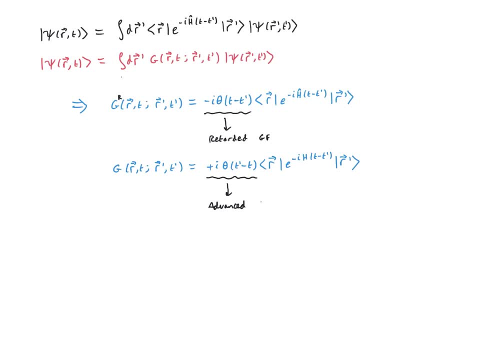 And these advanced Green's functions are often denoted by the superscript a. In this case we assume that the wave function on the left-hand side, here psi of r and t, occurs at a time before the wave function psi of r primed and t primed. 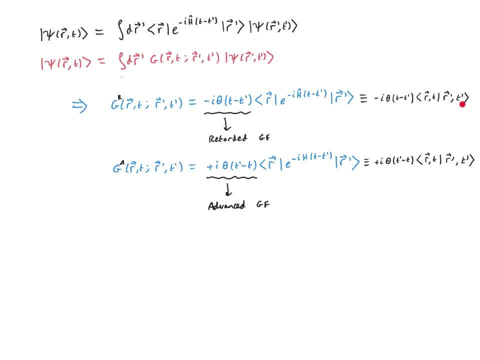 We can express these in the following way: in terms of these brackets, We see, therefore, that the Green's function Is basically associated to the probability amplitude of finding a particle in a state r and t, given that it started at r primed and t primed. 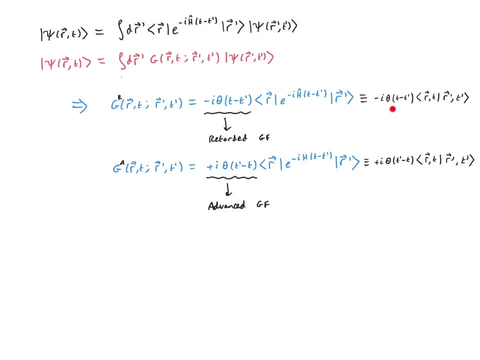 The retarded Green's function is the one where t is greater than t primed, and the advanced Green's function is the one where t primed is greater than t. So for the retarded function we start off in the state r primed and t primed. 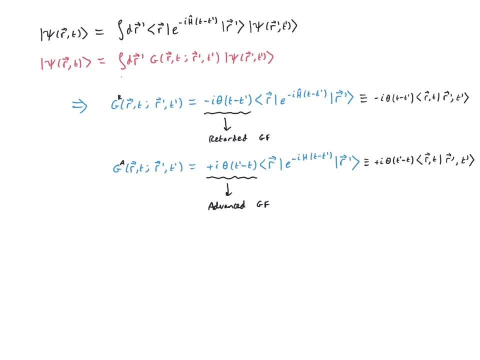 We move forward in time to r and t Now. I want to emphasise here that so far we've been considering the dynamics of a system with a single particle. However, in condensed matter physics, we're usually interested in systems of many particles. 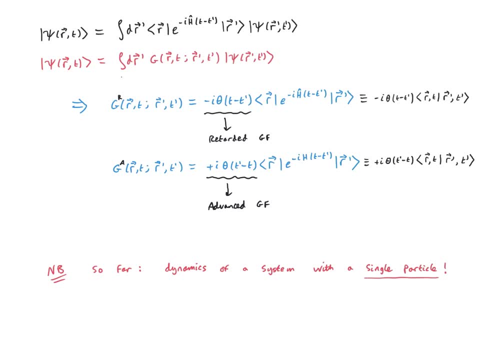 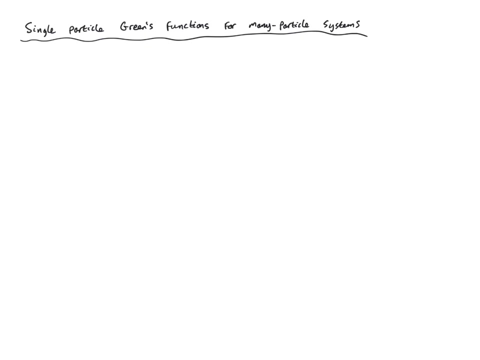 In fact, in the thermodynamic limit we'd have a very large number of particles- 10 to the 23 or so. So we need to be able to generalise this theory of Green's functions to systems involving many quantum particles. For the remainder of this lecture, and also in the coming lectures, we'll now focus on 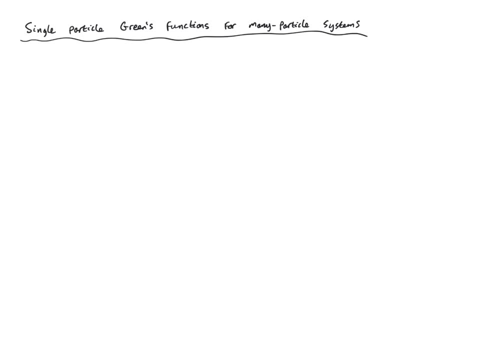 the single particle Green's functions. but for many particle systems, In many particle physics we'll adopt the same Green's function philosophy that we discussed on the previous slides, but we will need to generalise some of the concepts. Green's functions will describe the dynamics of electrons in many body quantum systems. 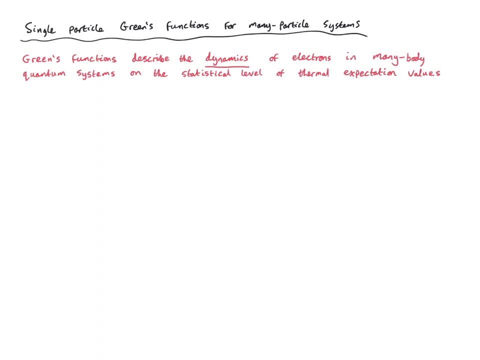 not on the individual level of single electrons, But on the statistical level of expectation values. We will see that these Green's functions are really the workhorse of many body quantum mechanics and they're very, very powerful indeed. We will see that single particle Green's functions only contain part of the full information. 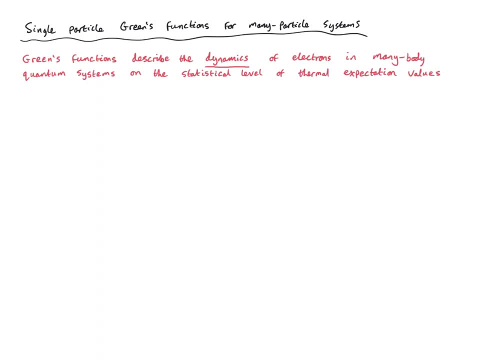 contained in the wave function. However, the information that they do contain tells us a lot about the system and, in fact, are closely related to various experimental observables of interest. We know that there are various different types of single particle Green's functions, but 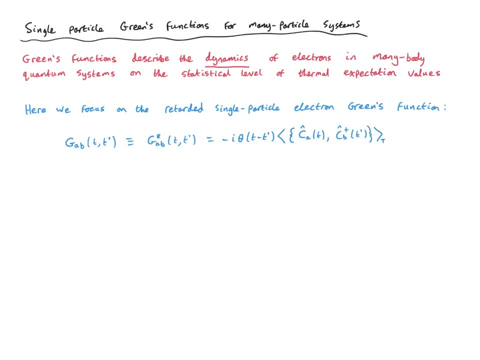 the one we'll consider in this lecture course will be the retarded single particle Green's functions for fermions. I will define it GAB of t and t'. t and t' here are the time labels and a and b are the orbital or site labels. 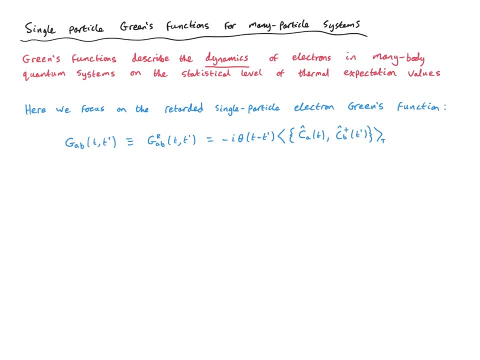 We're going to propagate an electron from site b to site a. To emphasise that this is the retarded Green's function, One can add this superscript r here However often. I will just drop this and assume that whenever you see a Green's function like 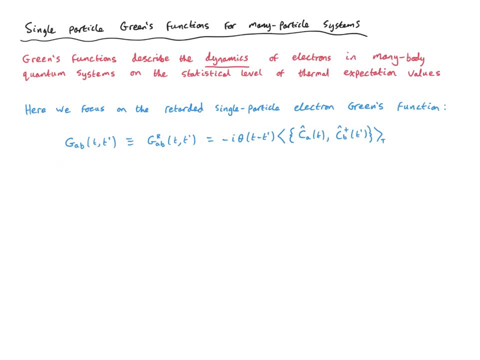 this. I'll be talking about the retarded Green's function. unless otherwise stated, The retarded Green's function is defined on the right hand side. here It's minus i theta of t minus t primed. This of course means that t has to be greater than t primed multiplied by the thermal expectation. 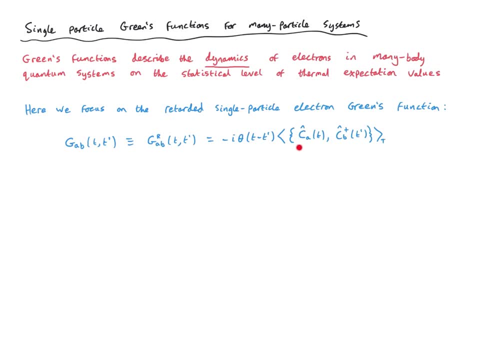 value of some operators, The operators, The operators, The operators. these inside here are the anti commutator of CA and CB dagger, evaluated at time, t and t primed respectively. This might seem like a rather complicated and abstract object, But we will be discussing the physical implications of this in the coming slides. 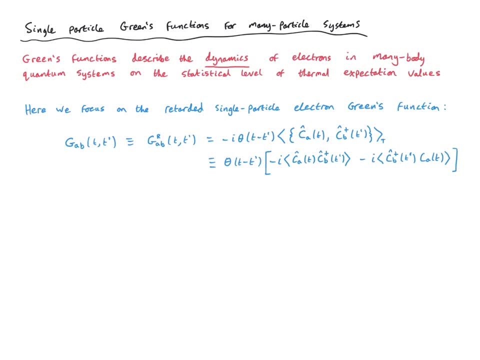 Writing out this anti commutator here I see that we have the sum of two terms. The first involves the thermal expectation Value of CA at time t and cb dagger evaluated at t primed, whereas the second expectation value has the 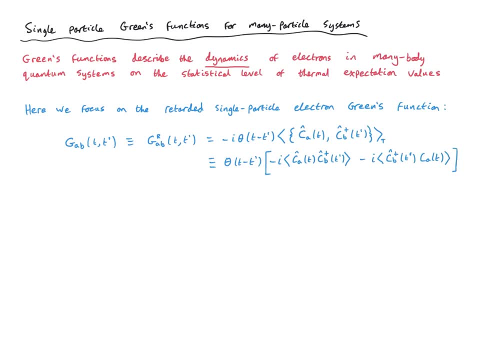 order of these operators switched. We have cb dagger evaluated at time t, primed, and ca evaluated at time t. And of course, in quantum mechanics the order of these operators matters even more so here because they have different time labels. We will denote each of these two terms as so-called 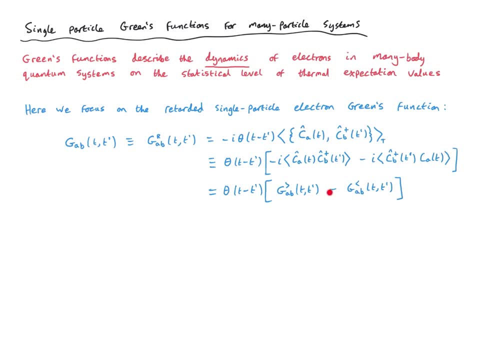 keldisch greens functions. We call the first term g greater and the second one minus g lesser. These are denoted by the greater than sign or the less than sign in the superscript here. Specifically, these keldisch greens functions are defined as: g greater is minus i times the. 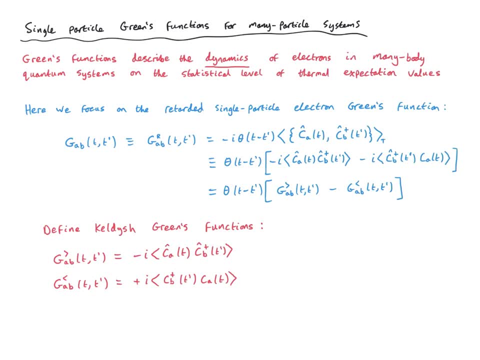 thermal expectation value of ca of t times cb dagger of c t primed, whereas g, lesser, is a greater value of ca, greater than cb dagger of t. So this is called the keldisch greens functions plus i times the thermal expectation value of Cb dagger evaluated at time t-primed, times Ca of t. 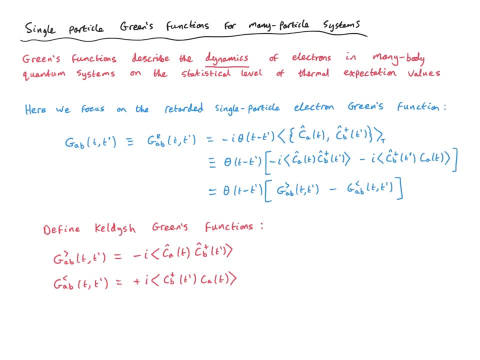 Notice that in these definitions we don't see the time ordering. There is no theta function That is pulled outside of the bracket here in the definition of the retarded Green's function. Apart from this decorative factor of minus i and plus i, here we can easily see what these Green's functions mean. 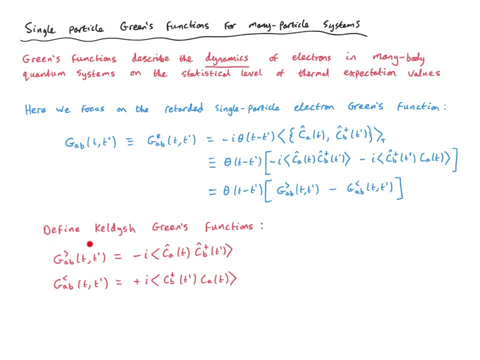 The physical interpretation of this G. greater is the probability that if I put an electron into the many-particle system at position or orbital b at time t-primed, then I can take the electron out at position or orbital a at time t. Notice that this does not have to be the same electron. 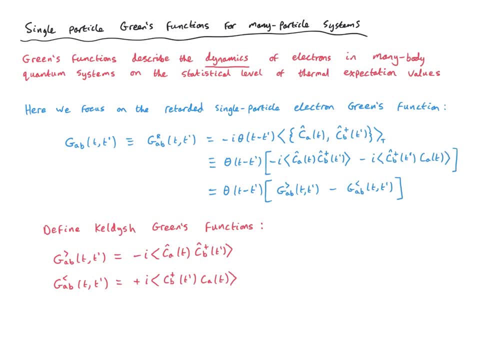 This is simply the overall thermal expectation value for such a process. Likewise for the G lesser, It's the probability that I can take out an electron at orbital a at time t and put one in in orbital b at time t-primed. 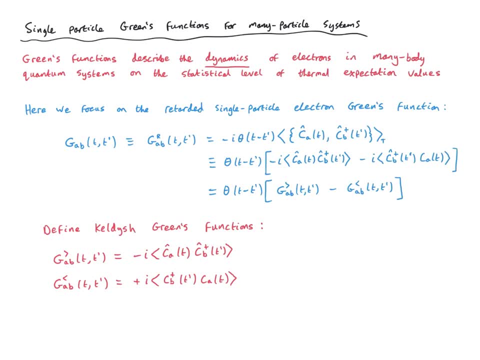 And again, here there is no time ordering. t can be after t-primed or t can be before t-primed. The order of t and t-primed is not specified in these Keldysh-Greens functions. 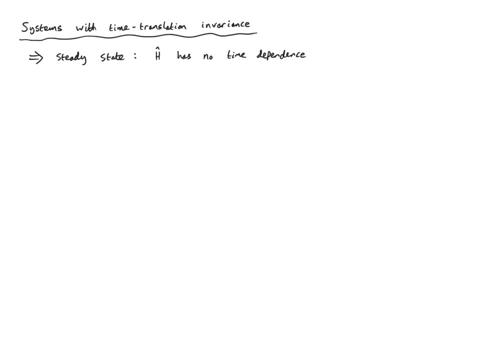 Let's now take a look at the special case of systems with time translation invariance. This means that we have a special case of systems with time translation invariance. This means that we have a steady-state situation. The Hamiltonian does not have a time dependence. 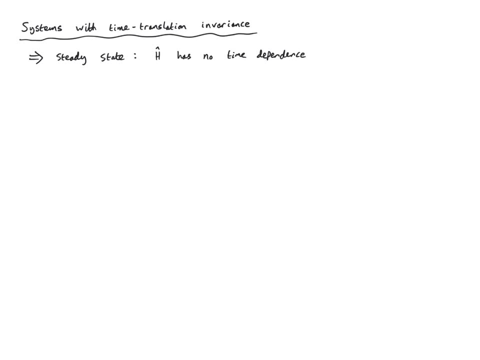 Obviously, this is a special case, but it's rather a common case and it's something that we're going to be studying a lot in this lecture course. Of course, one can have a non-equilibrium steady state, but more commonly we'll be discussing systems at thermal equilibrium. 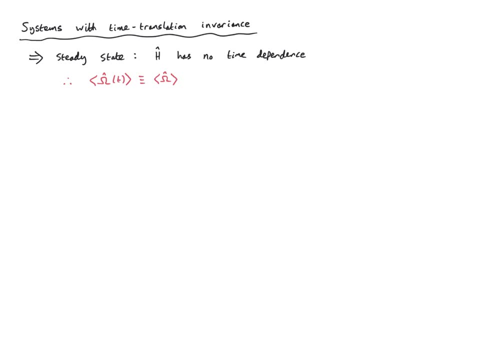 This means that the thermal expectation value of some operator evaluated at time t is static. It doesn't depend on the time at which you evaluate the expectation. However, it's a little more subtle when we're talking about the Greens functions, because we have two time variables. 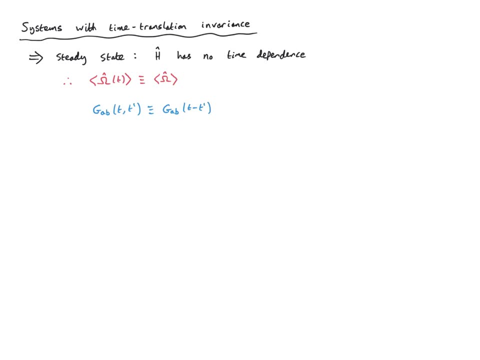 This tells us that the Greens function gab of times t and t-primed must depend only on the time difference between t and t-primed. So from now on, in this case we'll write gab of t minus t-primed. 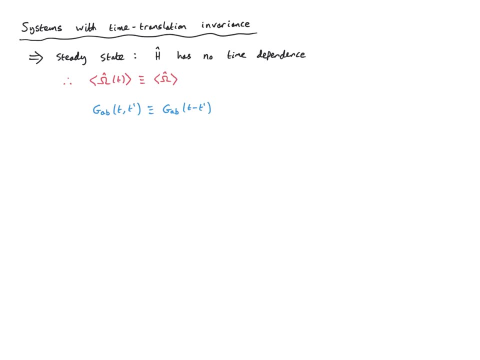 This is because the Greens function corresponds to a correlation function involving operators acting as a function of time. This is because the Greens function corresponds to a correlation function at times t and t-primed Because of the property of time translation invariance in the system. 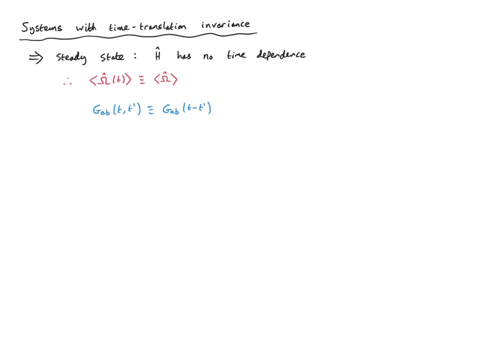 I can slide t and t-primed simultaneously backwards and forwards in time and still get the same answer. However, the correlation will depend on the time difference between t and t-primed. There will very naturally be a difference in the correlation between events separated by a short amount of time. 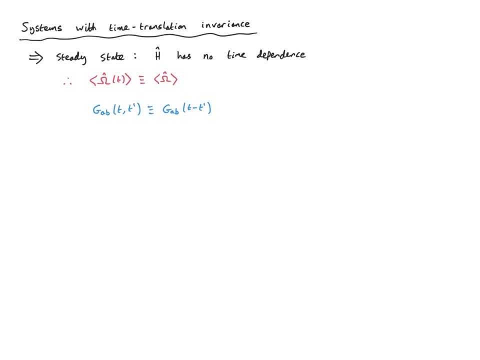 and events separated by a large amount of time. Indeed, since we can slide t and t-primed, at times t and t-primed, if we slide t and t-primed backwards and forwards in time and still get the same answer. 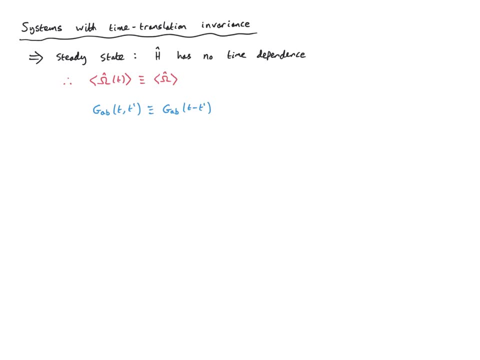 why don't we simply choose t-primed to be equal to zero? This then gives us that the Greens function, gab, is a function simply of the time t. In terms of the fundamental definition of our retarded Greens function, we can then write that gab of time t is equal to. 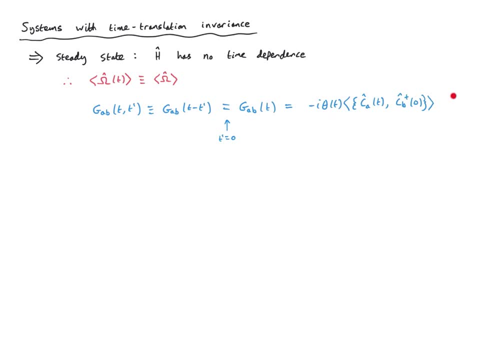 minus i. theta of t times the thermal expectation value of the anticommutator of ca, evaluated at time t, and cb dagger, evaluated at time zero. And just recall here that theta of t is the Heaviside step function, which is equal to 1 when t is greater than or equal to zero. 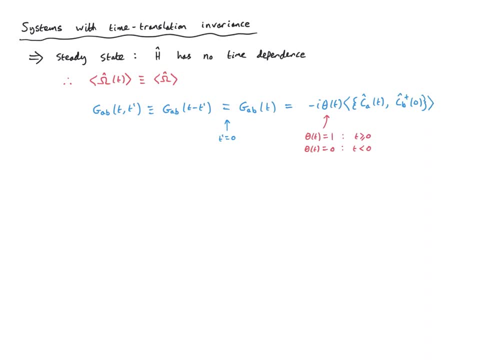 but theta of t is equal to zero when t is less than zero. Also, note that we can write cb dagger evaluated at time zero simply as cb dagger. We can drop the time label if t is equal to zero. That was all for the retarded Greens function. 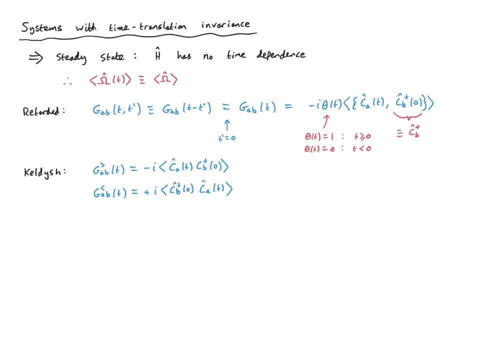 but we can now write cb dagger and we can similarly define the Keldysh components in the same way where we set t primed explicitly to zero in our time translation invariant system. In most of what follows we're going to be considering these equilibrium situations. 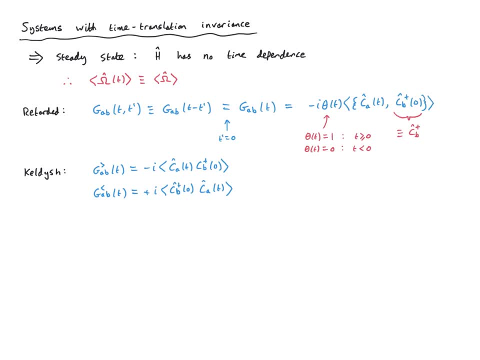 where the Hamiltonian has no explicit time dependence. The system will then have a natural time translational invariance and the corresponding Greens functions will be functions of a single time variable. You should just bear in mind that this time variable t corresponds to the difference in time. 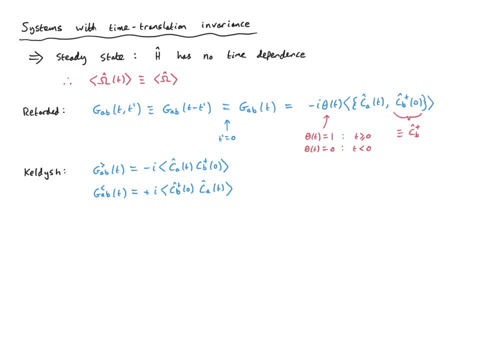 for the action of our two operators in the Greens function. Later on in this lecture, however, I will do one example of a system with an explicit time dependence, where the Greens functions then depend on two time variables, But for now let's just stick with the simplest case. 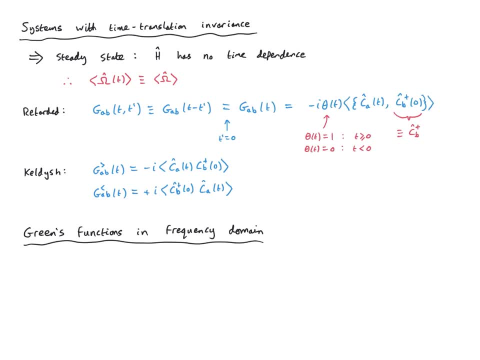 In this case we can naturally look at the Greens functions not in the time domain but in the frequency domain. There are actually some subtleties here due to whether we take the Fourier transform or the Laplace transform, and subtleties to do with the convergence of integrals. 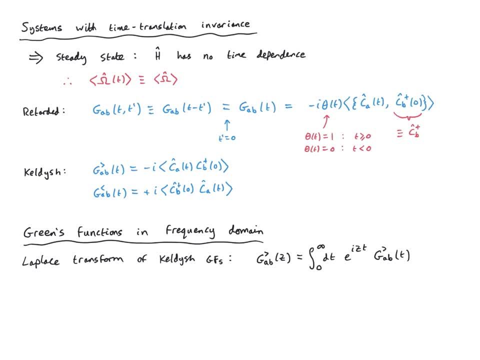 Let's define the Laplace transformation of the Keldysh-Greens function as g ab of the complex variable. z is equal to the integral dt from zero to infinity, of e to the i zt of the Greens function, g ab as a function of time. 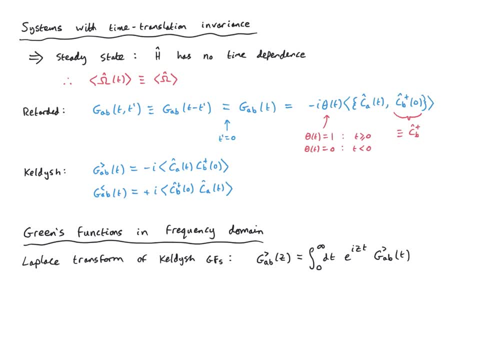 I've written this one down explicitly for g greater, but this exact same equation also holds for this. Here the complex variable z is defined as omega plus i delta, where omega and delta are pure real and delta in particular is greater than zero by definition. 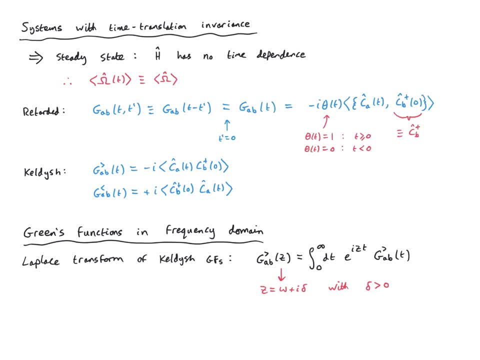 This is needed to ensure the convergence of these integrals. as we'll see shortly, The Laplace transformation of the retarded Greens function g ab of t is very similar, Since the retarded g ab of t is equal to the integral dt from 0 to infinity of t. 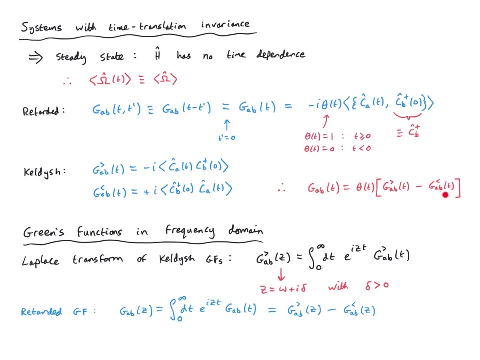 which is equal to theta of t, g greater of t minus g lesser of t. when we do the Laplace transformation, this theta of t doesn't matter, because we're already going from zero to infinity anyway. The time is always positive within this Laplace transformation. 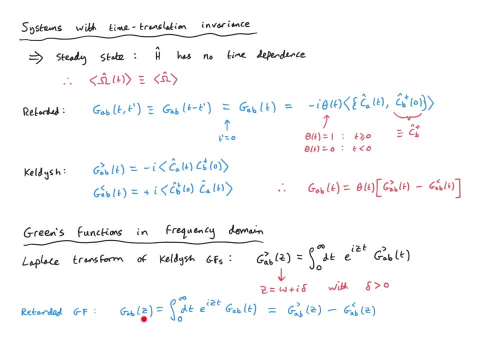 Therefore we can simply write that the retarded g ab of z is equal to g greater of z minus g lesser of z. Everything here is a function of the complex variable. z is equal to omega plus i delta, which is equal to omega plus i delta. 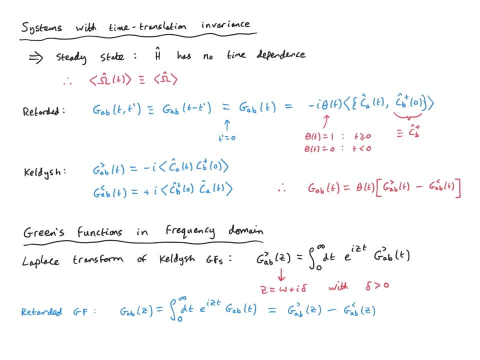 So how does this relate to Greens functions in the frequency domain which would be obtained by doing a Fourier transform? Well, the Fourier transform is defined as the integral dt from minus infinity to plus infinity, of e to the i, omega, t times. the Greens function g ab in the time domain g of t. 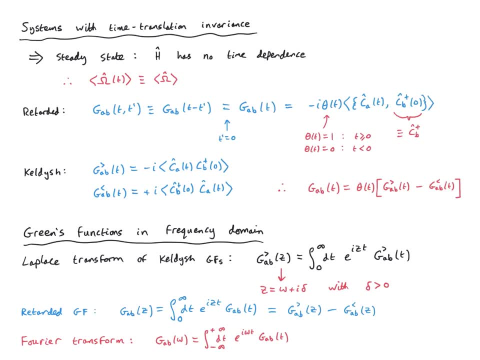 This would give the Greens function in the frequency domain g ab of omega. However, the definition of the Greens function in the time domain g ab of t, as defined in this equation, has, in the definition of it, this theta function, theta of t. 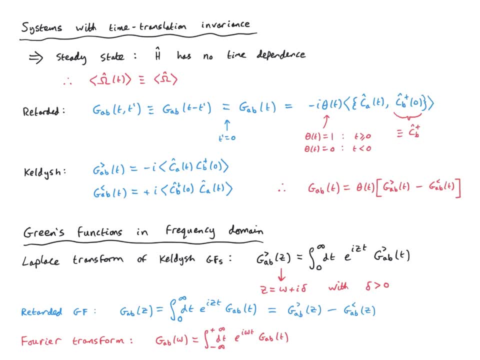 So when we insert that into this expression, it will of course kill half of this integral and we'll end up only with the integral dt from zero to plus infinity. This means that the Greens function in the frequency domain g ab of omega is very closely related to the integral dt from zero to plus infinity. 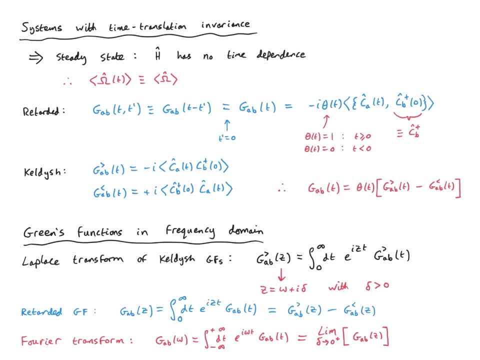 to that which we obtained by the Laplace transformation. GAB of z. GAB of z, of course, is a function of the complex variable omega plus i delta, with delta defined as being positive. Therefore, we can make the connection between GAB of omega and GAB of z by simply taking the 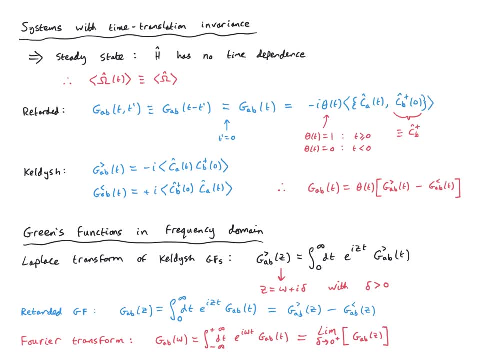 limit of the latter as delta goes to zero. However, since delta is defined as being positive, we have to take this limit of delta goes to zero plus. That means that delta remains positive, but it can become infinitesimal. In the end, we obtain the Fourier transform of the Green's. 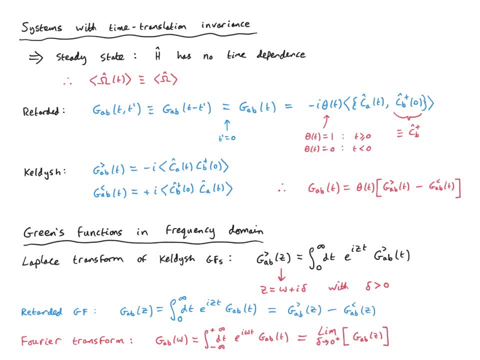 function in the frequency domain. This might seem rather convoluted and unnecessary. However, we'll see explicitly shortly that we cannot simply do a regular Fourier transform of these Green's functions because the integrals don't converge. We actually need to include an. 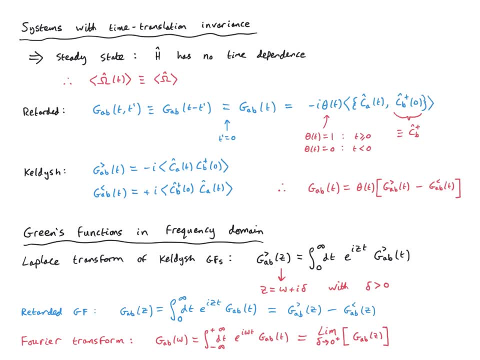 infinitesimal limit of delta goes to zero plus i delta, which is the limit of delta, goes to zero plus i delta. We can then define the Fourier transform by simply taking the limit of the imaginary part of z to zero, while keeping it infinitesimally positive. This is an example. 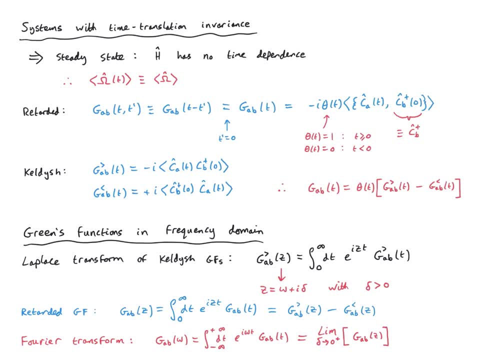 of so-called analytic continuation. We define G in terms of the complex variable z, with the positive imaginary part. G is therefore defined everywhere in the upper half complex plane. but then we examine the behavior of the Green's function G as we approach the real axis and send. 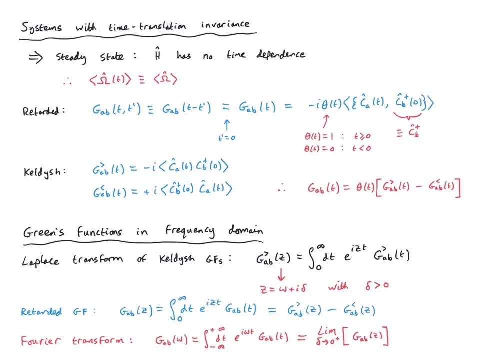 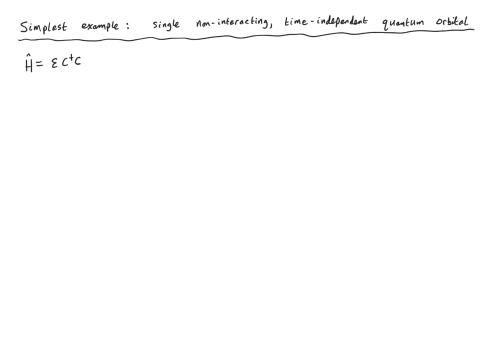 delta to zero, while keeping it positive. We therefore obtain G of omega, which is a function of real frequency, omega. Let's now have a look at an explicit example. In fact, let's take a look at the simplest possible example of a single, non-interacting and time-independent quantum. 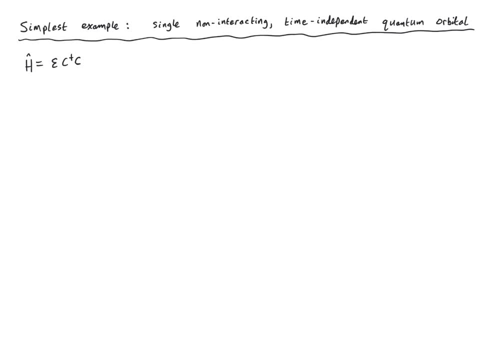 orbital. The Hamiltonian h-hat is a simple, non-interacting and time-independent quantum orbital. The Hamiltonian h-hat reads simply: epsilon c, dagger c, where epsilon here is the level energy for the single orbital. In the occupation number basis we have eigenstates. 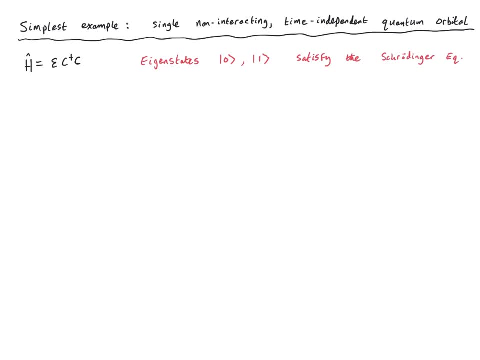 zero and one corresponding to the situation with no electrons or a single electron in our quantum orbital. And of course these satisfy the Schrodinger equation: h psi equals e psi. Specifically, h acting on the zero state gives us an eigenvalue of zero. 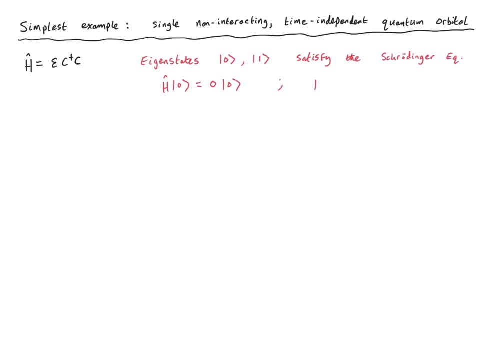 times the zero state back again, whereas h, acting on the one state, gives us epsilon times the one state back again. So the energies are simply zero if it's unoccupied and epsilon if it's occupied. Epsilon can therefore be understood as the single particle energy or local potential energy. 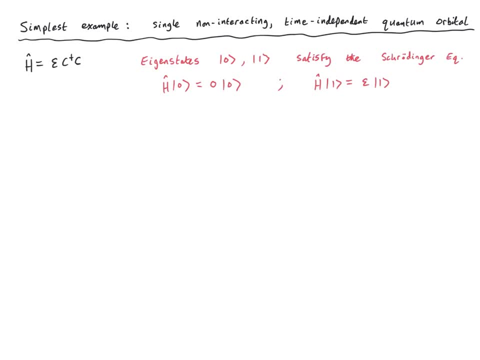 for this quantum orbital. Notice here that the Hamiltonian does not have an explicit time dependence. Therefore, our Green's function is a single particle energy or local potential energy for this quantum. orbital. Notice here that the Hamiltonian does not have an explicit time dependence. 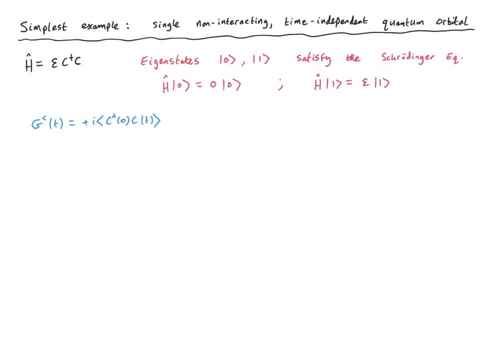 although the plutonium biomass will represent 2.2 함�� participations, We'll only involve relative time differences. Let's take a look at the lessor Green's function g. lessor of t. This is defined … as plus i times the thermal expectation value of the c dagger operator. 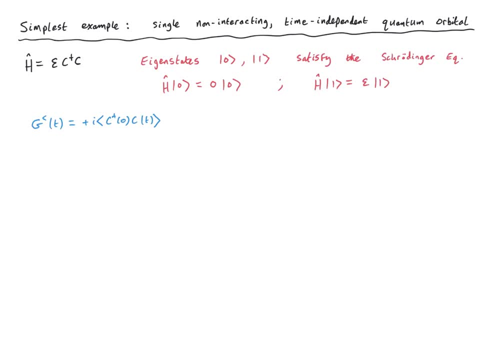 acting at time zero and the c-operator acting at time t. So how do we compute such an expectation value? Well, here let's recall that the time evolution of an operator, a hat, in the Heisenberg picture … is given by …. 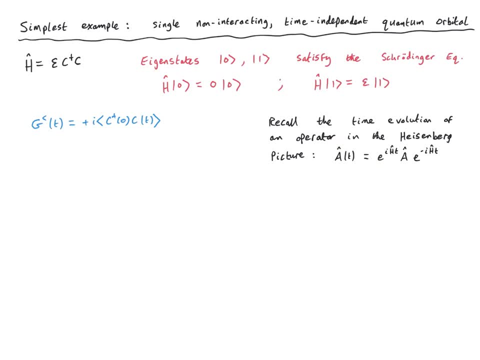 hat of t is equal to e to the iht times a times e to the minus iht, and here a hat is the time independent version of the operator for a time independent Hamiltonian h hat. We can therefore write that the g lesser greens function is plus i times the expectation value of a time independent. 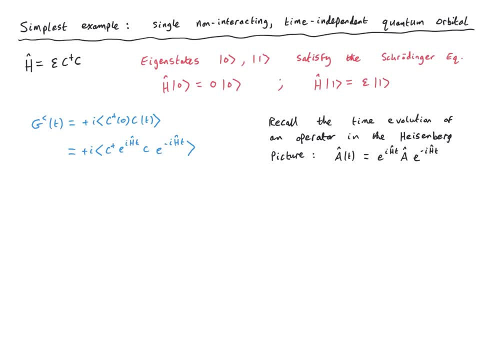 operator c: dagger times e to the iht times a time independent operator c times e to the minus iht. Next we need to calculate this thermal expectation value. Now we should recall that the thermal expectation value of some operator, a hat, within statistical mechanics is given by 1 over z times. 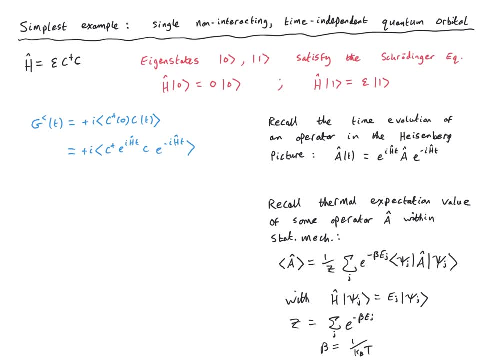 the sum over eigenstates j times the Boltzmann weights e to the minus beta ej. times the sum over eigenstates j times the Boltzmann weights e to the minus beta ej. times the matrix element of the operator a sandwiched between the eigenstates psi j. Here we have the. 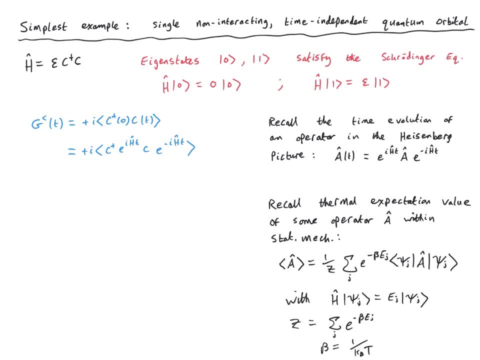 Schrodinger equation h psi is equal to e psi. In particular, if I act with the Hamiltonian on an eigenstate, psi j, I get the eigenstate back again. times the energy ej. This is the energy ej that is featuring in the Boltzmann weights. here in our statistical sum The factor z is, of course 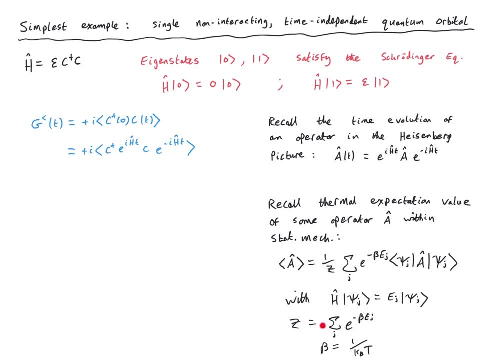 the partition function, which is simply the sum over all of these Boltzmann weights. It's basically normalising this probability distribution. Finally, beta is the so-called inverse temperature. It's just 1 over kB T, with kB the usual Boltzmann. 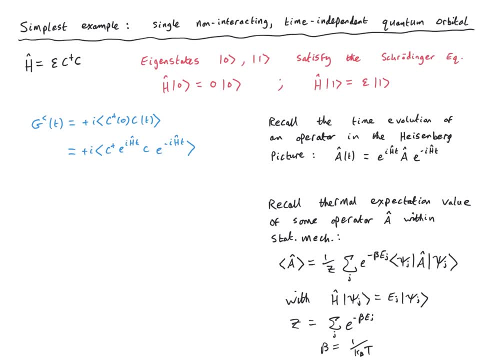 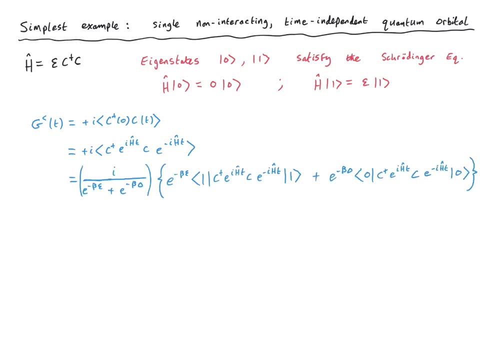 constant. So now we have all of the ingredients to simply go ahead and calculate by hand this G lesser greens function. So, putting all of this together, we have the following: First, we have this factor of i in the original definition divided by the partition function, which is the 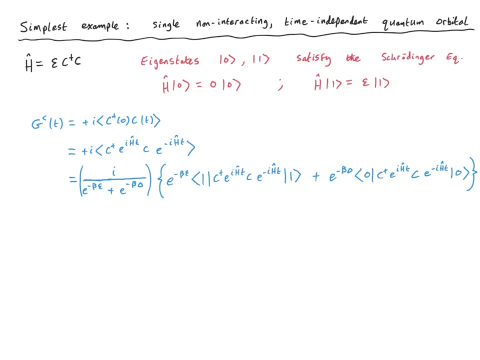 sum of the Boltzmann weights. And then we have the factor of i in the original definition, which is the sum of the Boltzmann weights, That's e to the minus beta epsilon, plus e to the minus beta zero, because we have two eigenenergies, zero and epsilon. Then we have the sum of two terms for 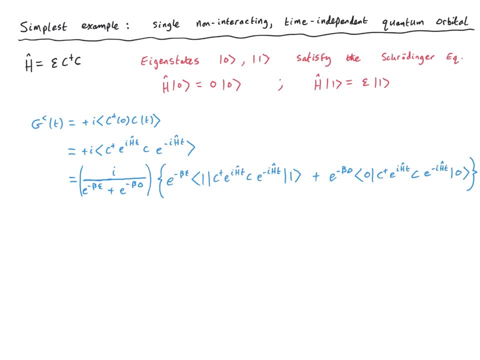 the two eigenstates. Each of these is weighted by its own Boltzmann factor. The first one, involving the occupied state, involves the Boltzmann factor e to the minus beta epsilon. The second one, involving the state zero, involves the Boltzmann factor e to the minus beta zero. The operators. 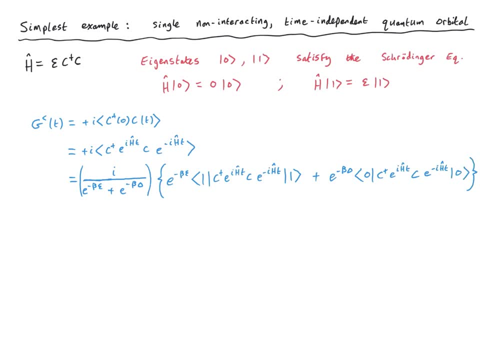 inside these matrix elements are the same. It's C dagger, e to the iHT C and e to the minus iHT. We can already make a simplification here, because e to the minus beta zero is of course simply 1.. 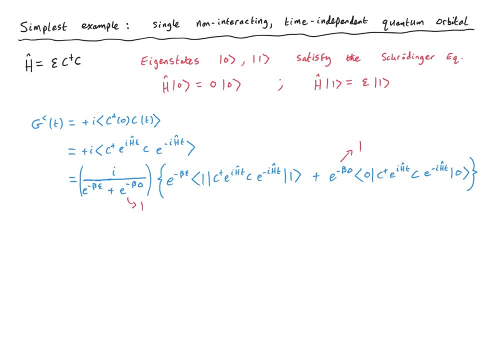 We can also immediately evaluate e to the minus iHT acting on the 1 state or e to the minus iHT acting on the zero state. That's because this exponential operator here involves a Hamiltonian and we're working in the eigenbases. The first of these terms gives us e to the minus i epsilon T. 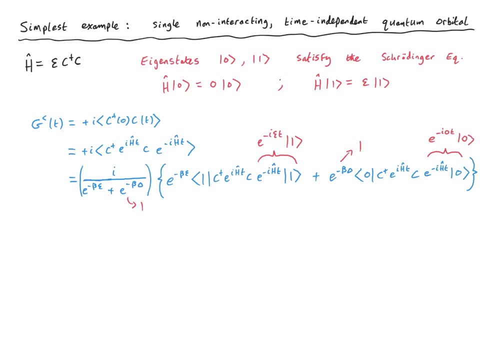 acting on the 1 state. That's because, of course, the 1 state is an eigenstate of the Hamiltonian, whereas the second one gives us e to the minus, i zero, T, And again this factor is, of course. 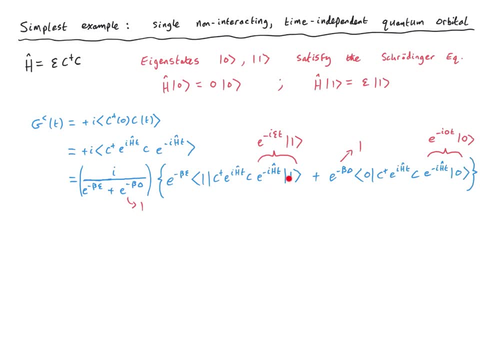 just 1 in the end. If you're curious about the way that these exponential operators act and why I'm allowed to simply replace the operation of the Hamiltonian on the eigenstate by simply the eigenvalue. you can think about just expanding this exponential as a Taylor series. 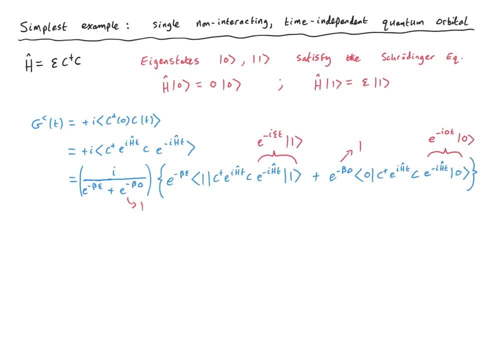 in powers of the Hamiltonian. Anyway, the resulting factor e to the minus i epsilon T or e to the minus i zero T, these things are of course just pure numbers and commute through the rest of these operators, so I can collect those exponentials together as common factors. 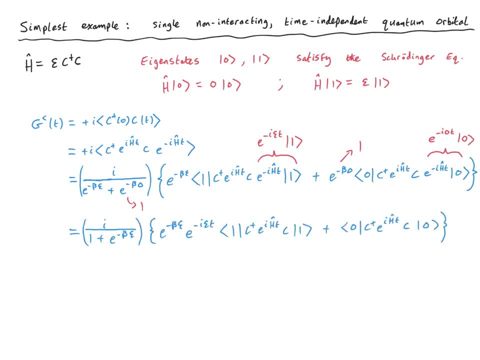 Then I obtain this expression. Importantly, we see here that this second term is essentially equal to zero, because we have the action of the annihilation operator C acting on the already empty state. So this gives us zero and kills that whole second term. 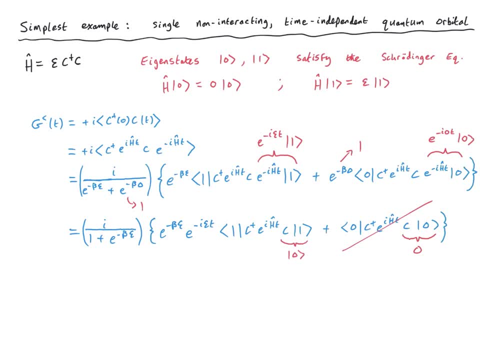 Likewise, in the first term, we have the annihilation operator C acting on the occupied state, which of course gives us the zero state. Furthermore, we can then act on this zero state by the exponential operator e to the i h T, and that will give us e to the i zero T. 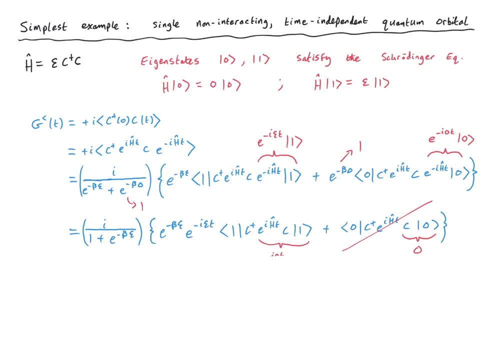 in this case e to the i. zero T is of course just a factor one, That's a number that can be commuted outside of the matrix element, which gives us overall the C dagger operator acting on the empty state, which of course gives us the occupied state. So in the end we're looking 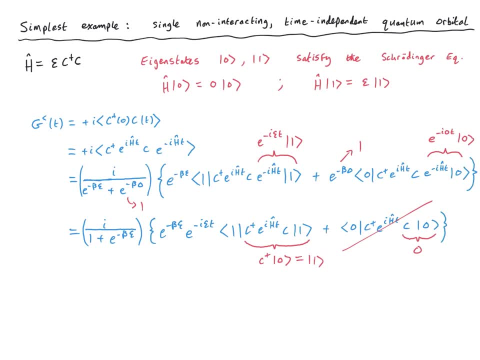 at the overlap of the one state with itself, and that object is simply equal to one. So overall, the difference between the two is that the C dagger operator is acting on the empty state and the one state is acting on the empty state and the one state is just a number. So that's the difference. 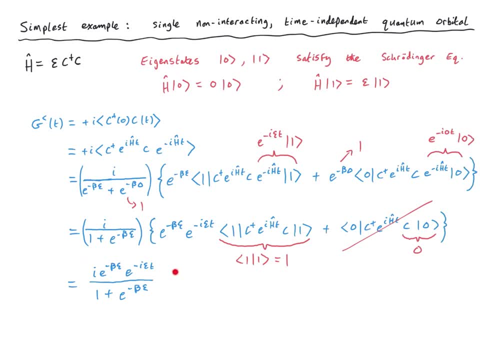 between the two. The lessor-Greens function as a function of time is simply i, e to the minus beta epsilon times, e to the minus i epsilon t divided by the partition function 1 plus e to the minus beta epsilon. If I then multiply this expression top and bottom by e to the plus beta epsilon, then I get this. 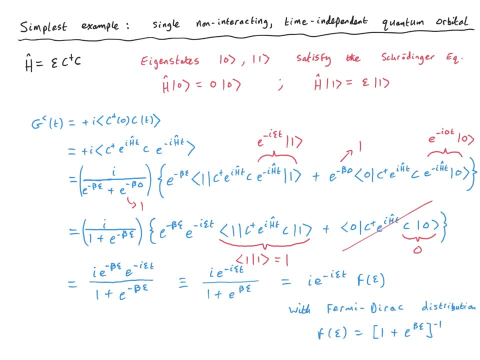 slightly simplified form. Furthermore, this can be expressed in terms of the Fermi-Dirac distribution f of epsilon, defined in the usual way as 1 over 1 plus e to the minus beta epsilon. As we know, the Fermi-Dirac distribution controls. 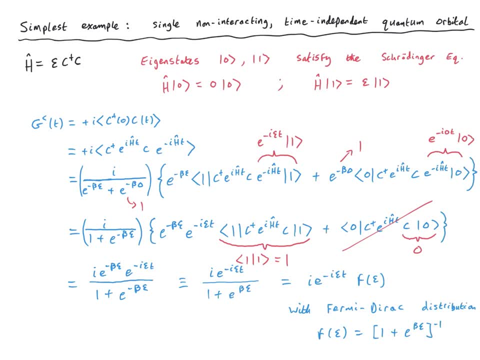 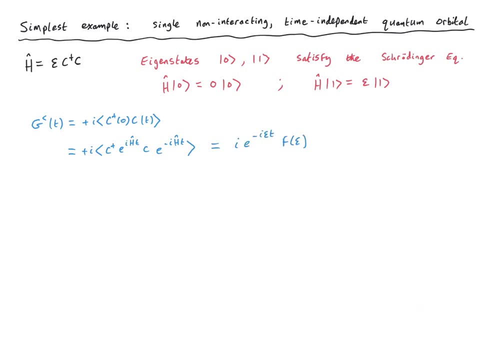 the thermal occupation of the orbital and we see it here entering in the g-lesser Green's function. So we see from this explicit expression that the Green's function g-lesser of t is actually something that is periodic in time. That is because of this factor e to the minus. 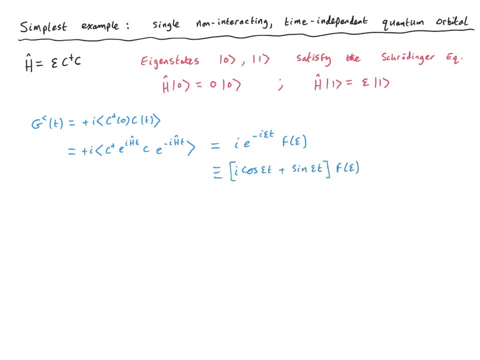 i epsilon t, Using Euler's relation to write e to the i theta as cos theta plus i sine theta, we can then express g-lesser of t in this way. The imaginary part of g-lesser of t as a function of time is therefore simply a cosine. The amplitude of the oscillation is simply the. 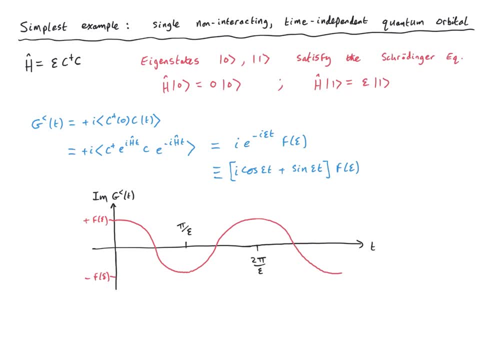 Fermi function. we see it goes between plus f of epsilon to minus f of epsilon and the time period is 2 pi upon epsilon. We have a periodic structure to the Green's function and this goes on forever in time Before we discuss the corresponding. 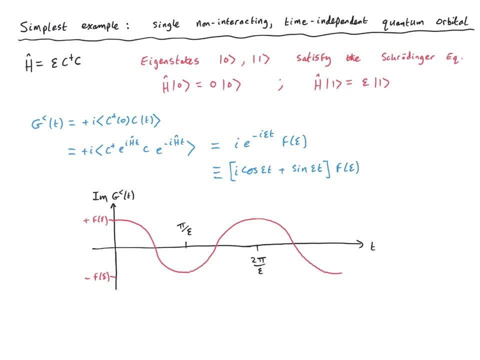 Fourier transforms and the Green's functions in frequency domain. let me make a comment on the equal times Green's function. If we consider again now the two times Green's function, g-lesser of t in t' but now we look at equal times, t' is equal to t. then that would have the explicit. 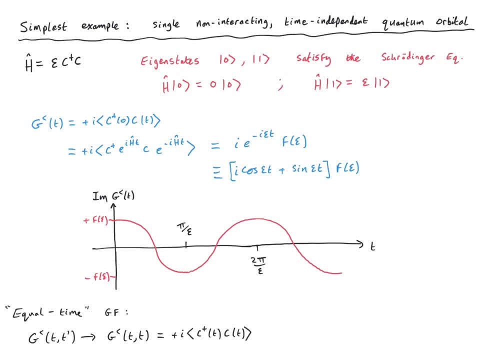 expression written on the right hand side here, Due to time and translation, invariance of the system, given our Hamiltonian, does not depend on time. we can evaluate this Green's function at any specific time and we can choose in particular. t equals zero, So in time-independent. 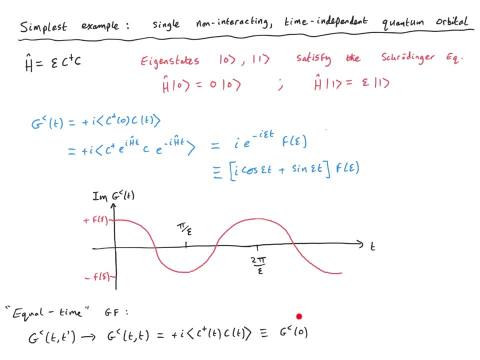 systems, the equal times Green's function is simply equal to the t equals zero Green's function. We can now go to our explicit expression for g lesser of t and set t equals to zero to discover that g lesser of zero is simply equal to i times the Fermi function f of epsilon. We can also see: 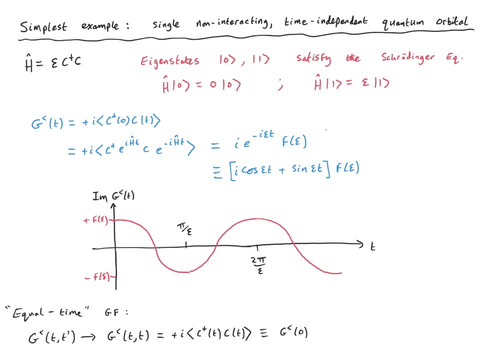 that from the graph here, The imaginary part of g lesser is equal to f of epsilon. However, g lesser of zero has another interpretation. Plugging t equals zero into this expression simply gives us the expectation value of c, dagger c. This is, of course, the expectation value of the number. 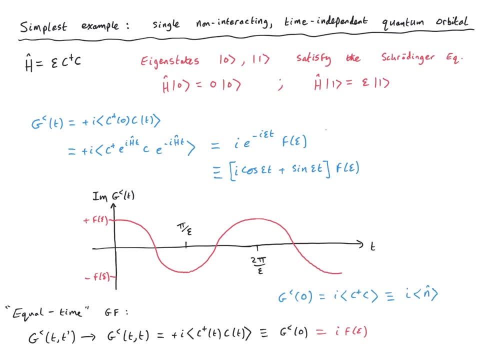 operator for our single site, We can write g lesser of zero, therefore, simply as i times the expectation value of the occupation of our site. So we see that we get the static expectation value of the operators. when we look at the zero time or equal time Green's function Furthermore, we recover the expected result. 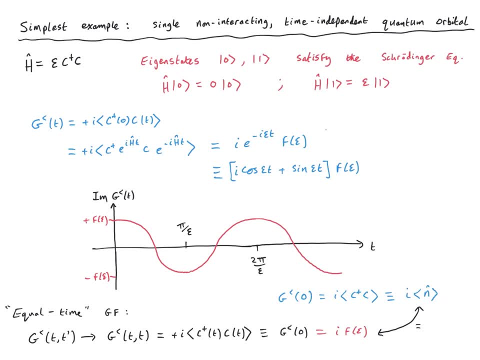 We see here, by equating these two expressions, that the expectation value of the occupation for our site is given by the Fermi function. This is precisely the meaning of the Fermi function: It's the thermal expectation value of the occupation of a quantum orbital. So all of this makes good. 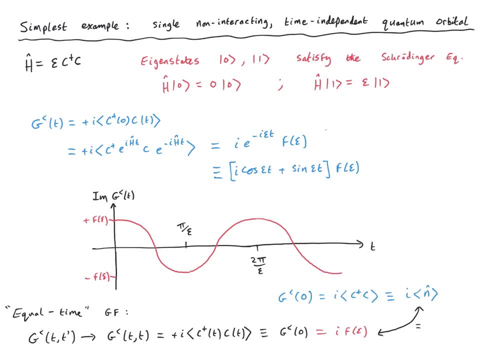 sense. Okay. so what about the Green's function in the frequency domain? Well, in the time domain, we see that we have an oscillatory function with a well-defined frequency. Because we have a single frequency to the oscillation, we expect in the frequency domain a delta function. So let's see. 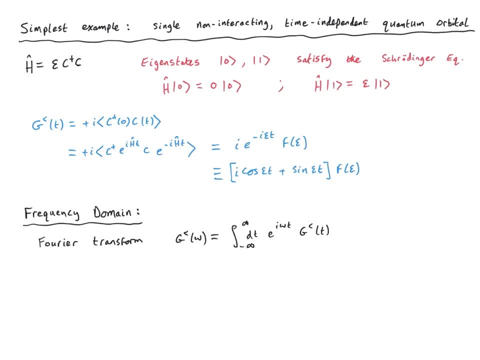 how that works out mathematically. First of all let's examine the naive Fourier transformation. So we have a function of f of epsilon times. the integral dt over all time g lessor of omega is equal to the integral dt over all time of e to the i omega t of g lessor of t By substituting in: 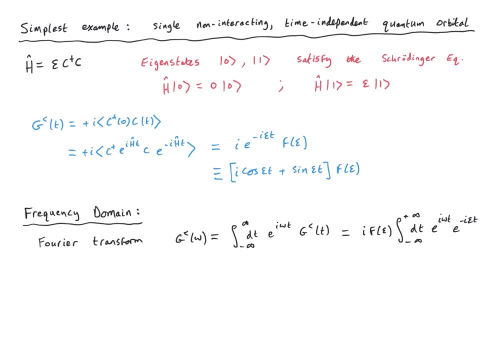 this explicit expression for the g lessor Green's function in the time domain, we obtain the following: This looks like a rather simple integral. We have: i times the Fermi function f of epsilon times the integral dt over all time times this factor coming from the Green's function e to the minus i epsilon t, Of course. 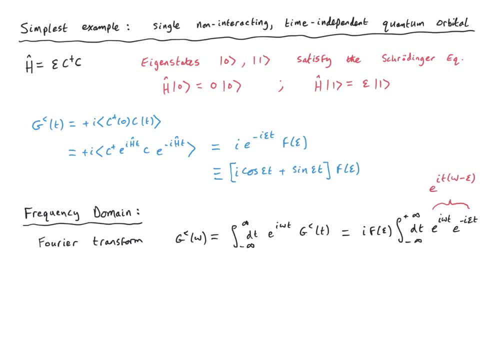 we can collect together these two exponentials here as e to the i, t multiplied by omega minus epsilon. And now we can simply do the integral. We obtain this object, which is then evaluated at t equals minus infinity and t equals plus infinity. And now we have to pause and think a little bit. 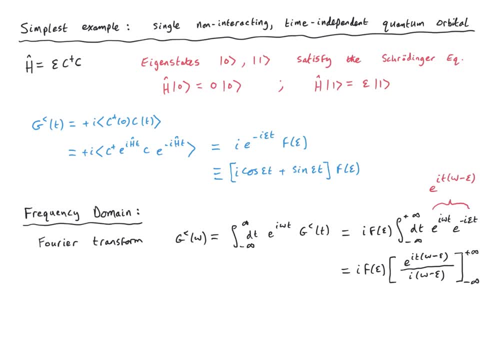 because there's some problems with this expression. The first giveaway that there's a problem is that downstairs we have omega minus epsilon. What happens when we want to evaluate the Green's function g of omega at the point omega equals epsilon? This would be undefined. 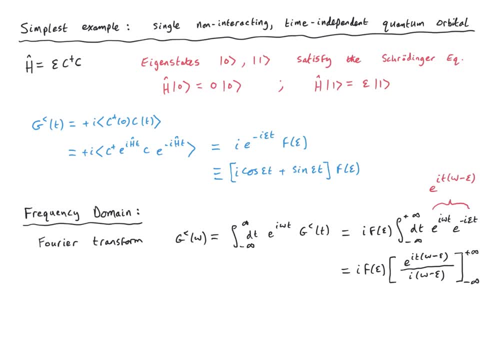 because we'd have a divide by zero problem. That's the first hint. The second hint that something's wrong is that we have to evaluate this integral at t equals minus infinity and plus infinity. But, as we already saw, e to the i, t, omega minus epsilon is an oscillatory function. 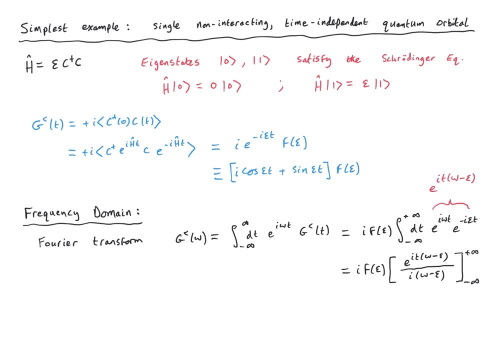 so we have to be a little bit more careful. What value do we assign it at? t goes to infinity or minus infinity? We could write e to the i t omega minus epsilon as cos t omega minus epsilon plus i sine t omega minus epsilon. But what value do we assign this at? t equals infinity. 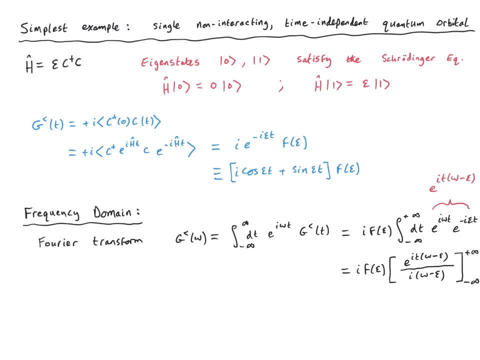 It's oscillating between plus and minus one. Naively, it might appear that this integral is actually undefined. However, we have to be a bit more careful. In theory of Fourier analysis, you might recognise the integral dt of e to the i, t, omega, minus. 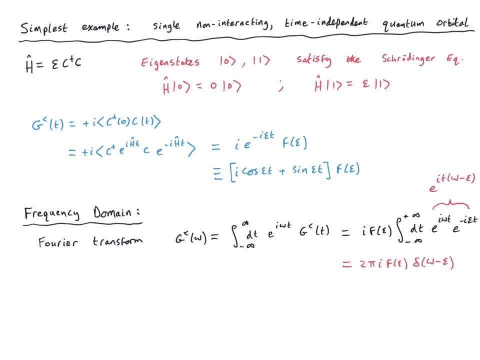 epsilon is actually the definition of the delta function, So we can actually write that g lesser of omega. for pure real frequency, omega via the Fourier transform is given by 2 pi, i fermi function, f of epsilon times the delta function, the Dirac delta, omega minus epsilon. 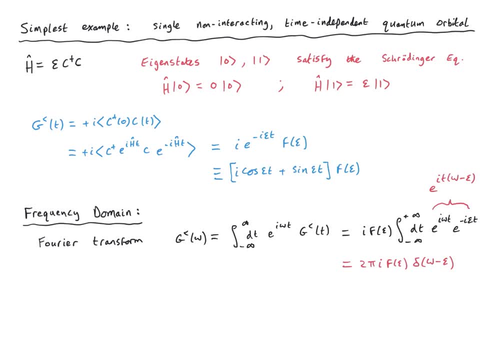 I'll return to this formulation a bit later. However, first let's look again at the Laplace transformation of g lesser of z. As before, the Laplace transformation for g lesser of z is defined as the integral dt from 0 to plus. 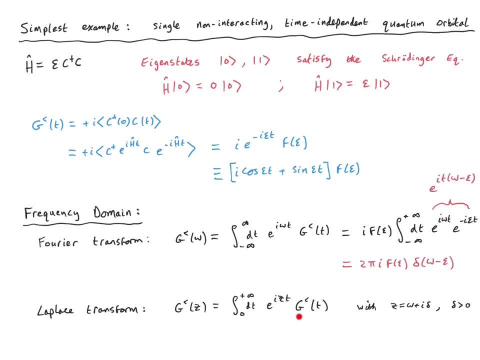 infinity, this time of e to the i z, t times g lesser of t. Here z is a complex variable, omega plus i delta, where both omega and delta are real and delta is taken to be positive. Well, going through the same steps as before, you obtain a very similar expression. 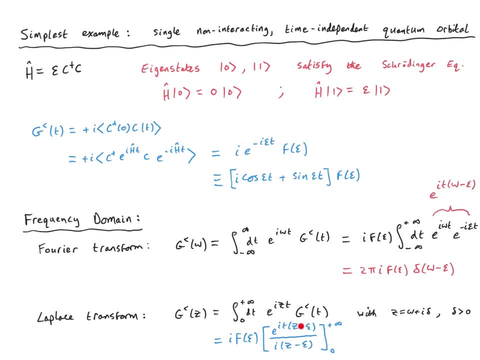 f of epsilon times e to the i t, z minus epsilon over i. z minus epsilon, evaluated between t equals 0 and infinity, The integral is well-behaved and convergent. First of all, let's look downstairs here. Now we have z minus epsilon on the denominator. 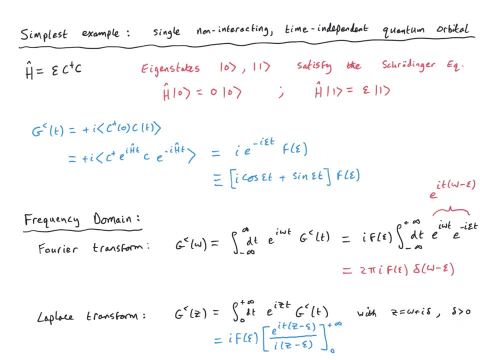 As long as that we have a finite imaginary part with delta greater than 0 here, this tells us that the denominator can never actually be equal to 0. That's because epsilon is real, so there's no divide-by-zero problem in this equation. 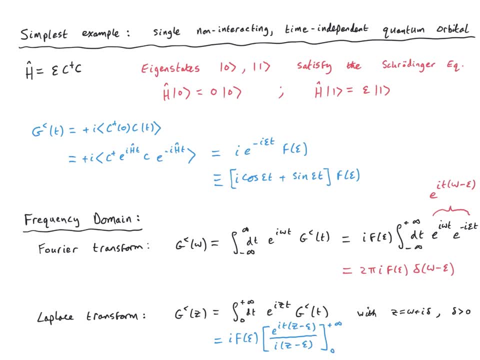 So let's have a look now at evaluating this definite integral at the two limits: t equals 0 and t equals infinity. Okay, so this lower limit here is obviously well-behaved because we plug in: t equals 0 there and the top is equal to 1.. What about in the case of t goes to infinity? Here we have z divided by a integral, plus a function of t equal to infinity. If we substitute explicitly 0 and 0, then we get a minus. While we're doing this now, let's instead look at the other limits. Let's first look at the definition of infinity. 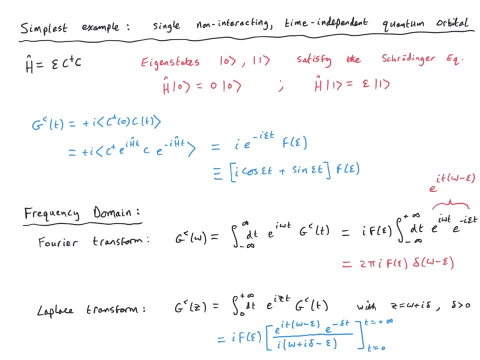 Let's take an example and see how this works. So this is the definition of infinity. So this lower limit here is obviously well-behaved, because we plug in t equals 0 there and the top is equal to 1.. If we substitute explicitly z equals omega plus i delta, then we obtain the following: 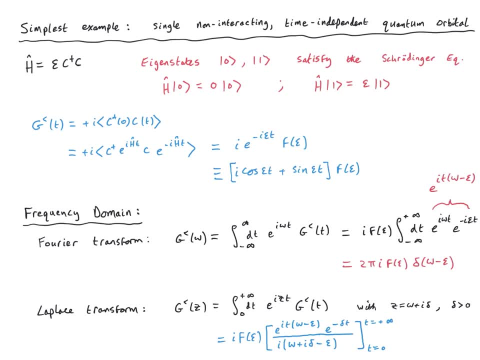 In particular notice that the plus i delta factor on the numerator becomes e to the minus delta t. And if delta is positive, as we've assumed here, then this factor will ensure convergence of the integral as t goes to infinity. This e to the minus delta t will exponentially suppress anything in this expression here as t becomes large. 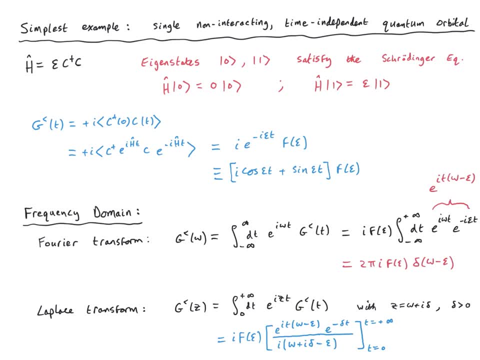 As we've already discussed, this first term is oscillatory and is bounded from plus to minus one. So this e to the minus delta t will certainly suppress those oscillations at large time, giving us a convergent solution to our problem. On the bottom we see explicitly that even if omega is equal to epsilon, 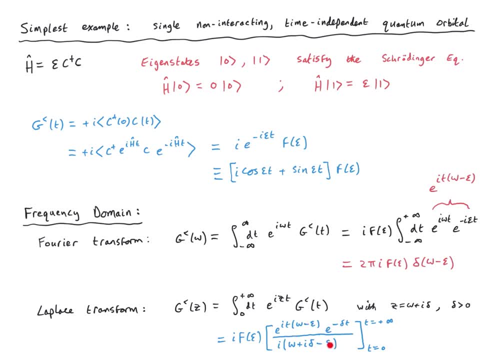 this will not be a divide by zero problem because we have a finite, So overall the integral converges, We have a well-behaved function. It evaluates to minus f of epsilon over z minus epsilon. Let me come back to the physical interpretation of this expression when we discuss the corresponding retarded Green's functions in the frequency domain. 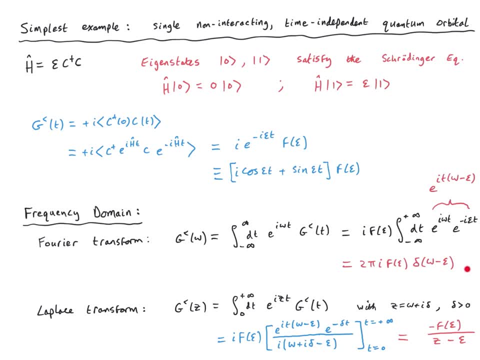 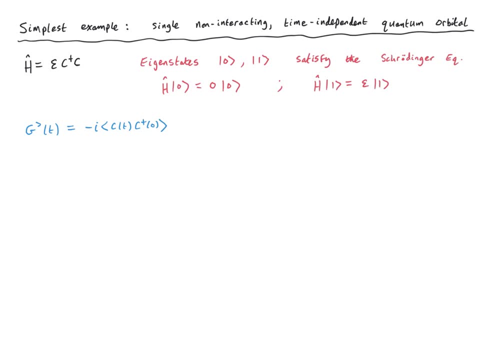 I will also discuss the relationship between the result for the Fourier transform and the result for the Laplace transform. So far, we've been considering the differential equation. We've been considering the G-lesser function. Now let's turn to the corresponding G-greater function. 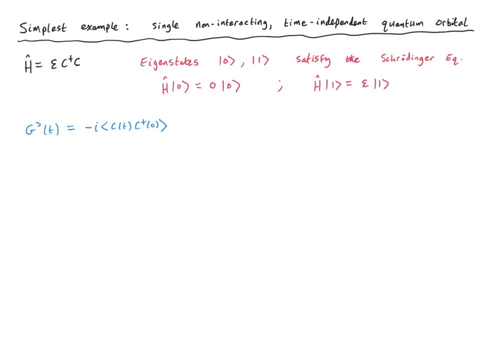 G-greater of t is defined as being minus i times the thermal expectation value of the operator c of t and c-dagger of zero. We can now evaluate explicitly this expression in exactly the same way as we did for the G-lesser. 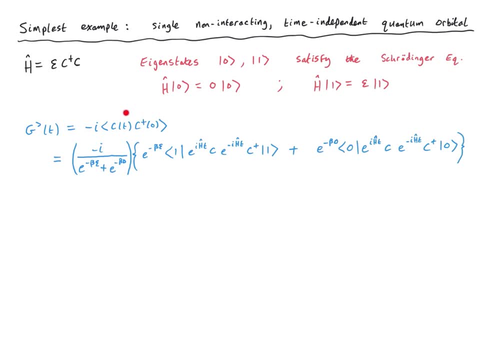 Using the previous definitions of the time evolution of the operator c of t. and also using the expression for the expectation of the time evolution of the operator c of t. and also using the expression for the expectation of the time evolution of the operator c of t. 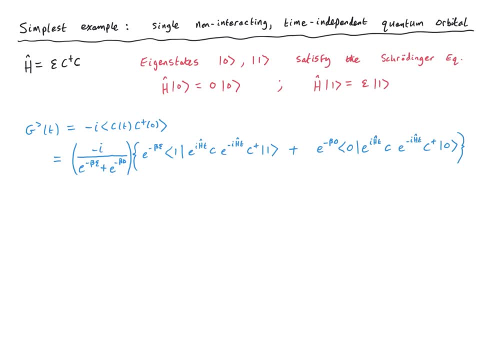 we obtain the following: This is exactly an analogy to the G-lesser function that we considered previously. As before, we can immediately make some simplifications. First of all, e to the minus, beta to 0 is 1 in both of these two factors. 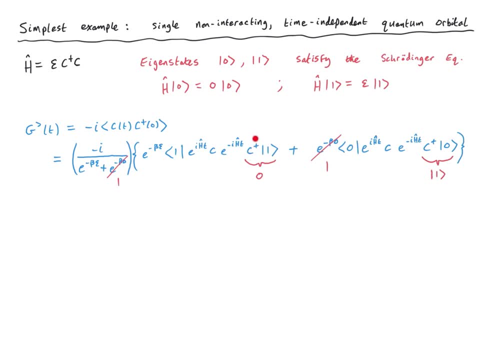 Also, we have c-dagger acting on the occupied state at this time and this is equal to zero, whereas in the second term we have c-dagger acting on the unoccupied state, which gives us twice the Greoy integrate gives us the one state. The expression for g greater of t therefore collapses. 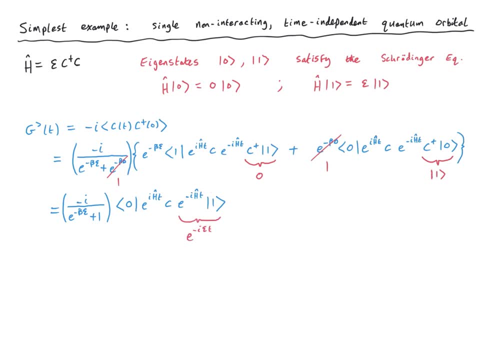 to this e to the minus i h t acting on the occupied state, of course gives us the factor of e to the minus i epsilon t times the occupied state back again. e to the minus i epsilon t is of course just a number commutes through these. 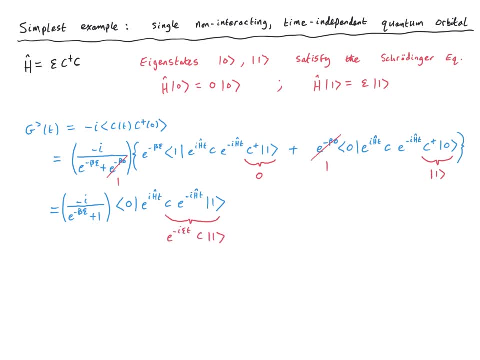 operators and we can collect it to the front of the expression. We can therefore write e to the minus i, epsilon t times c, acting on the one state. This of course just gives us the empty state. Then we act one more time with e to the plus i. 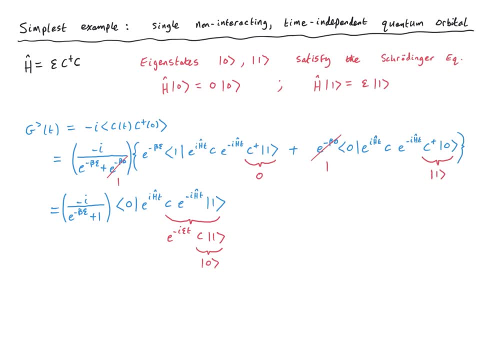 h, t on the empty state, which gives us a factor of 1.. And then we simply have the brackets of 0 with itself, which is 1.. So, collecting all this together, we have that g greater of t is equal to minus i times e. 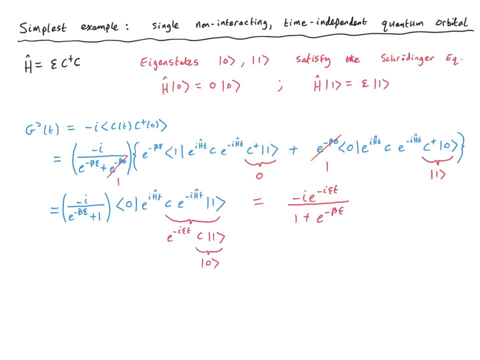 to the minus i epsilon t divided by 1 plus e to the minus beta epsilon. As before, we can now multiply top and bottom by e to the plus beta epsilon, and then I again recognize the Fermi function: 1 over 1 plus e to the beta epsilon. So in the end we see a slightly different expression. 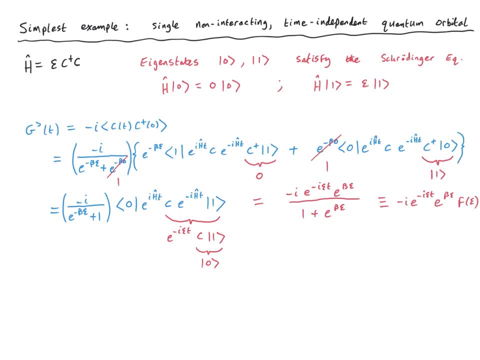 for g greater, We have a minus sign and this extra factor of e to the beta epsilon. In fact, with a bit more manipulation we can actually eliminate this factor e to the beta epsilon by expressing it in terms of the Fermi function. I will leave it as an exercise for you to prove that the g greater 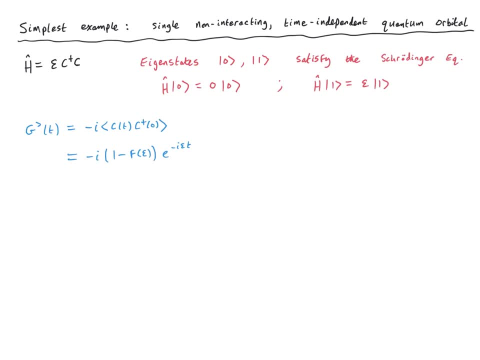 function can be written in this form as: minus i into 1, minus the Fermi function times the factor e to the minus i epsilon t. Now we can interpret the factor of 1 minus f of epsilon here as being the population of holes, If f of epsilon was equal. 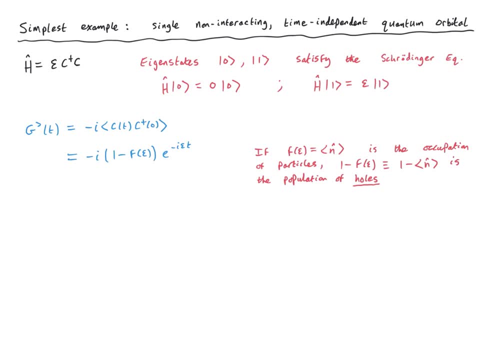 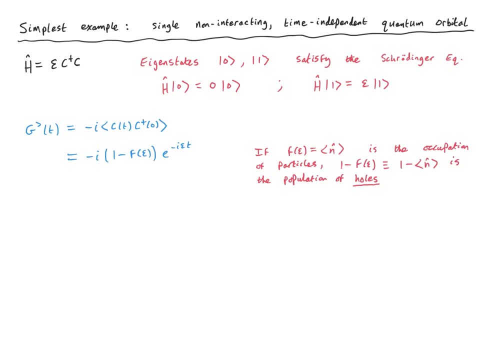 of particles. So 1-f is then the occupation of the holes. It might seem rather strange to talk about the population of holes, but it's simply a complementary way of counting things. We can either count the number of particles relative to zero occupation, or we can count the number of holes relative to an occupied site. 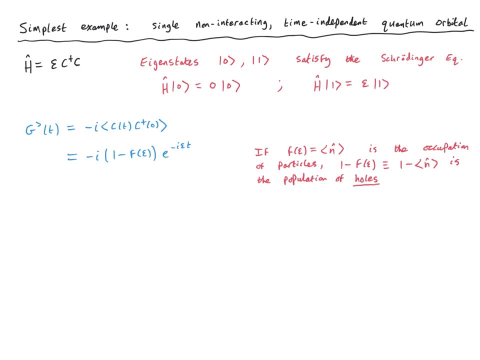 So we see that the g-lesser function is basically the Green's functions for the particles, and the g-greater Green's function is the Green's function for the holes. The imaginary part of g-greater of t therefore again has an oscillatory form, This time. 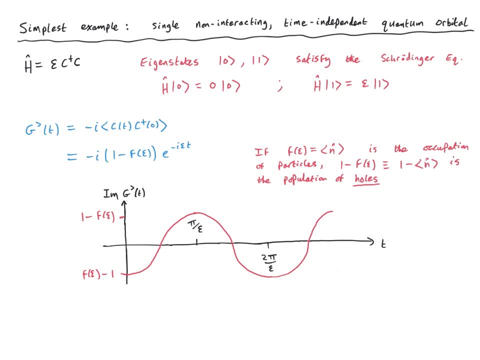 the amplitude goes between 1-f and f-epsilon-1.. Of course we see the same time period of 2 pi over epsilon for the oscillations. Let's now see how to calculate the time period of the oscillations. Let's now take a look at the Green's function in the frequency domain. As before, we'll 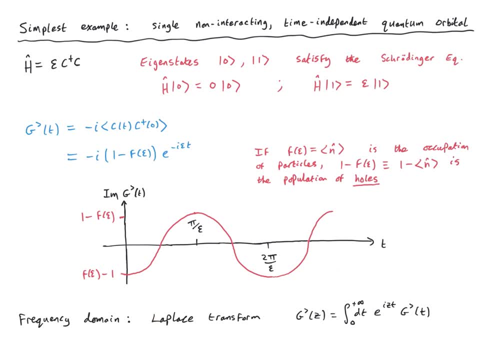 actually apply the Laplace transformation and relate g-greater of z to g-greater of t by integrating over time, from zero to infinity, of e to the i-z-t times, the time domain g-greater of t function, Following exactly the same steps as before. 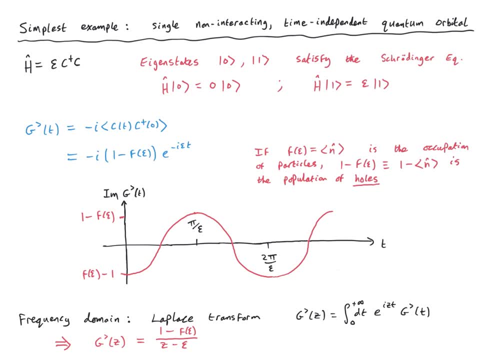 we obtain that g-greater of z is equal to 1 minus the Fermi function divided by z. Alternatively, we can perform the regular Fourier transform and in that case, very similar to the case of g-lesser, we obtain minus 2 pi i, 1 minus f of epsilon times. 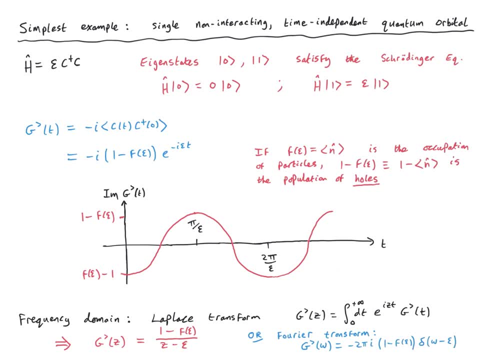 the delta function omega minus epsilon. These are two equivalent ways of performing the transformation, either to the complex argument z or to the real frequency omega. So let me now summarise: In the time domain we can perform the Fourier transformation. 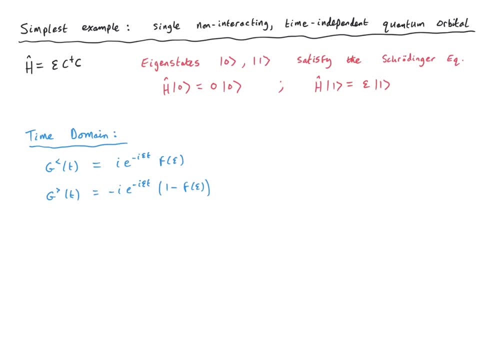 and in that case we obtain g-greater of z times the time domain, g-greater of t times the delta function omega minus f of epsilon In the time domain. for this simple example of a single non-interacting time-independent, 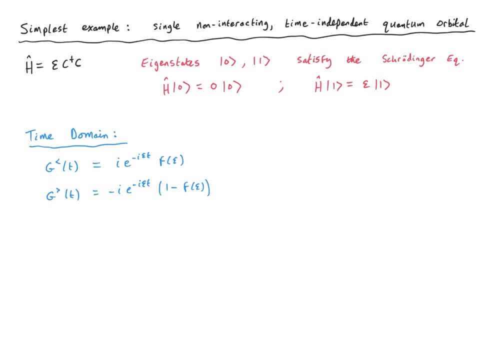 quantum orbital. we have g-lesser functions and g-greater functions. They're related to this factor e, to the minus i, epsilon t, and we have these Fermi factors f of epsilon entering In particular. we're now in a position to calculate the retarded Green's. 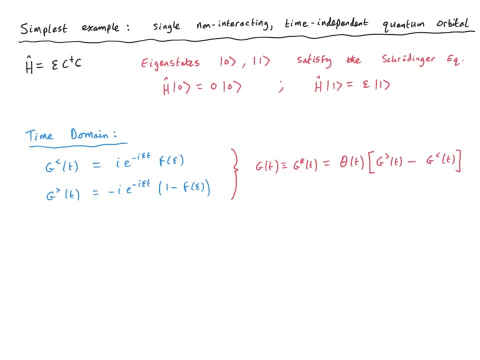 function g of t. As we showed earlier, this is simply theta of t, the heavy side step function multiplied by g-greater of z times the delta function g-greater of z. We can now simply substitute in our expressions for g-lesser and greater and find out an explicit 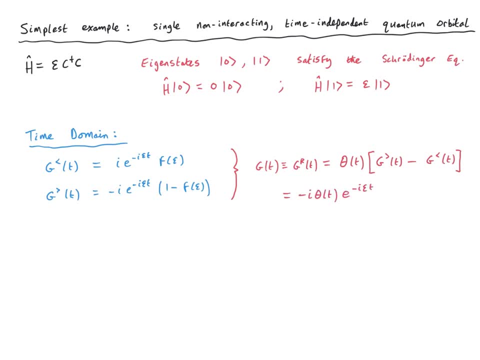 expression for g-retarded. When we do that, we find that g-retarded is simply minus i, theta of t, times e to the minus i, epsilon t. The Fermi functions exactly cancel out. This is very interesting because it tells us that g-retarded has no temperature dependence. Notice that, the temperature dependence. 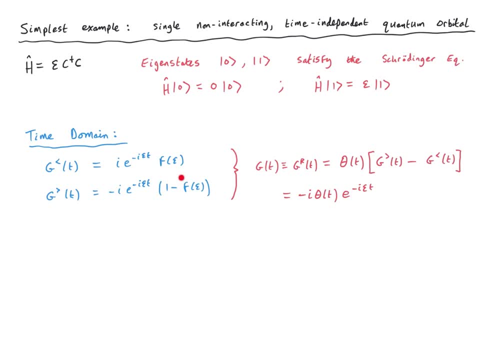 of our thermal expectation values entered entirely through these Fermi functions and they've cancelled out here. g-retarded has no temperature dependence for this non-interacting system. So our retarded Green's functions do not depend on the thermal or statistical occupation of our quantum orbital. 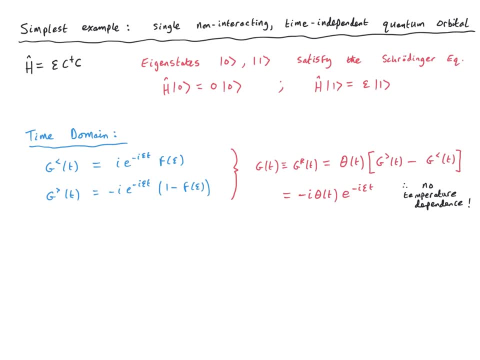 So what information does it contain? Well, to answer that question, let's have a look again at the frequency domain. In the frequency domain, and here I mean functions of the complex Z obtained by the Laplace transformation, we have g-lesser of z being minus f of epsilon. 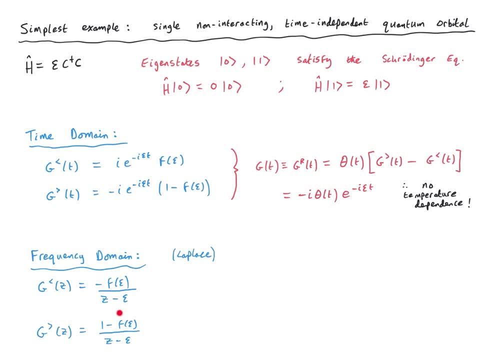 over z minus epsilon, whereas g-greater of z is 1 minus f of epsilon over z minus epsilon. The corresponding retarded Green's function in the frequency domain g of z is therefore g-greater of z minus g-lesser of z, as before, which of course gives us in this case 1. 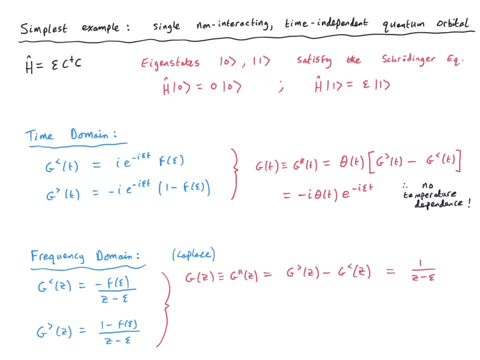 over z minus epsilon. Again we see that the Fermi functions cancel out. they drop out. we have no temperature dependence to the retarded Green's function In particular. we can now also relate the lesser and greater Green's functions to the retarded function. We find that g-lesser is equal to minus the Fermi function times g-retarded. 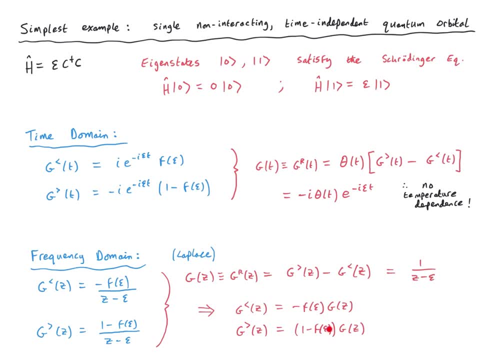 whereas g-greater is equal to 1 minus the Fermi function times g-retarded. These are actually related to the so-called fluctuation-dissipation theorem and are quite general. We can really apply very generally in any equilibrium system, as we'll see. 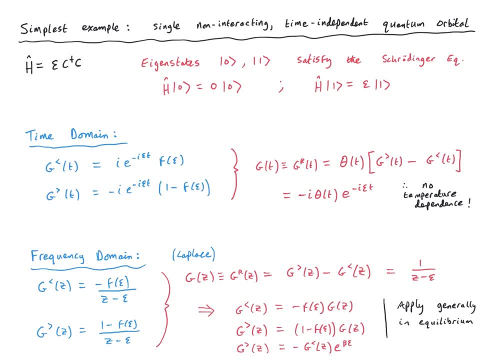 g-greater and g-lesser can of course also be directly related, and we find that g-greater of z is equal to minus g-lesser of z times the factor e to the beta epsilon. Note here that there is no simple relationship between g-retarded as a function of real frequency. 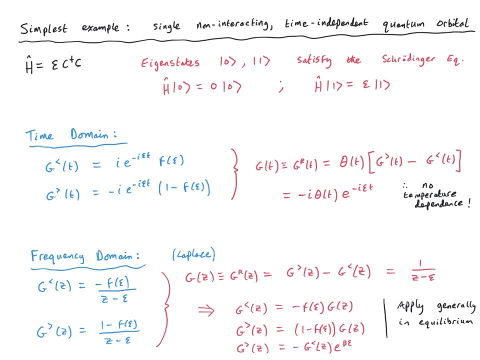 omega obtained by the standard Fourier transformation and the g-lesser and greater functions as a function of real frequency omega obtained by their corresponding Fourier transforms. And that is because, if we look at the definition of g-retarded in the time domain given here, 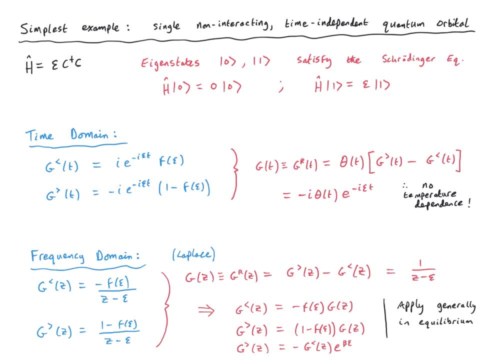 we see that it contains this extra theta function. So the Fourier transform of g is not simply equal to the difference of the Fourier transforms of g-greater and g-lesser because of this extra factor theta. But we'll see an alternative formulation for that shortly. 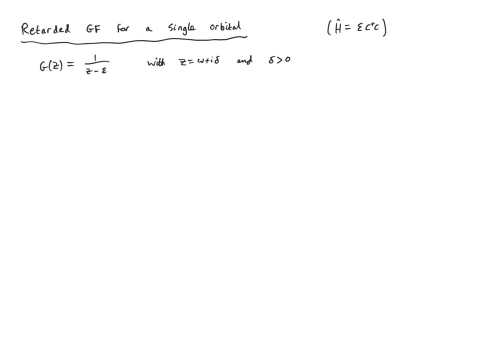 So let's now focus on the retarded Green's function for this single orbital. We've just derived that g is equal to 1 over z minus epsilon. with a complex z equals omega plus i, delta and delta positive. We can now look at the real and imaginary parts of g and we find the following expressions: 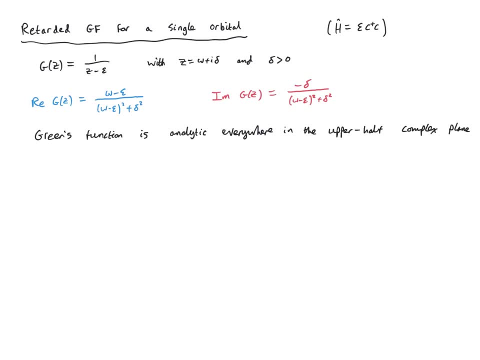 In particular. you'll see from these expressions that g is well-behaved and analytic everywhere for delta-greater And we say that the delta regularises these Green's functions In particular. I can write minus 1 upon pi of the imaginary parts of the Green's function. 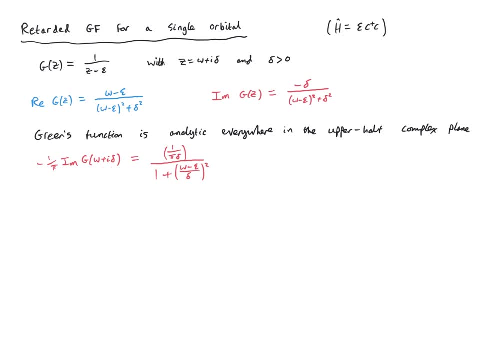 g. In this way, I write it as 1 over pi delta, all divided by 1 plus omega, minus epsilon over delta squared. This is the very definition of the Lorentzian function, centred on omega, equals epsilon and of width 0.. 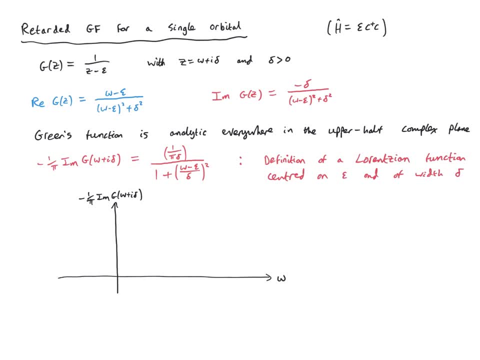 So let's now plot this function as a function of epsilon for a given delta. For a fairly large delta, we see the Lorentzian has a rather broad width. In fact, it is easy to show from this explicit form that the peak is located exactly at omega. 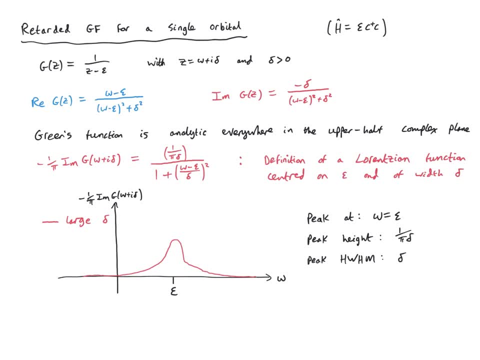 equals epsilon. the peak height is 1 over pi delta and the half-width at half-maximum of the peak is exactly delta. Therefore, as we go to a smaller delta, we see that the peak gets higher and it gets narrower, but is still centred on omega equals epsilon. 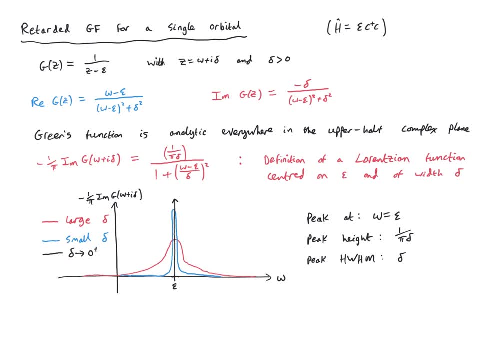 In fact, as delta goes to 0 but remains infinitesimally positive, this will turn into a delta peak, meaning that this has infinitesimal width and infinite height. In fact, the Lorentzian is a mathematically well defined approximation to the Dirac delta. 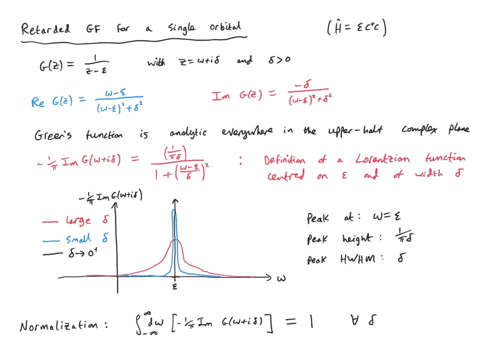 distribution. We can see that because principalarias form이�omo, tore, vịata, DNA, 부가 말 나, Joint γ and nogeme React forces. the normalization of the Lorentzian, which is the integral d, omega from omega, is minus infinity to. 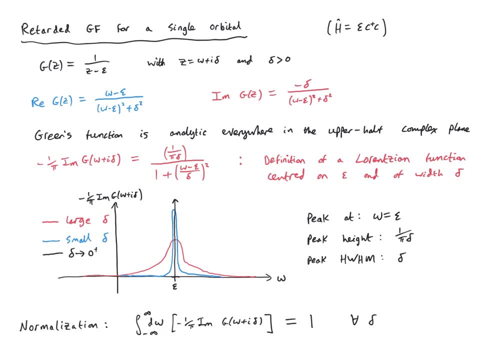 plus infinity of this object minus 1 upon pi of the imaginary part of g is equal precisely to 1, and that's independent of the delta. This means that if I were to integrate this red curve here, I would find an area under that curve of 1.. If I integrate the blue curve, I would find an area 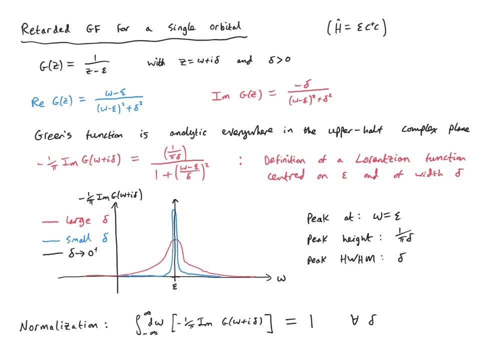 of 1, and indeed, as I send delta to 0,, keeping it infinitesimally positive of course, I still find that the normalization of that is equal to 1, and that's one of the important properties of the delta distribution. So we see that as we take the limit, of delta goes to 0 plus. 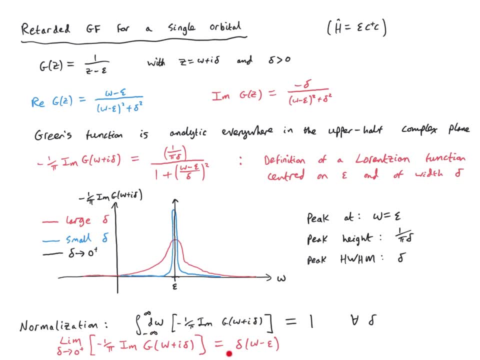 of minus 1 upon pi of the imaginary part of g, we see exactly the delta function of delta omega minus epsilon. This is an important quantity and we give it a name. We call it the spectral function. The spectral function a of omega is defined as being the limit. 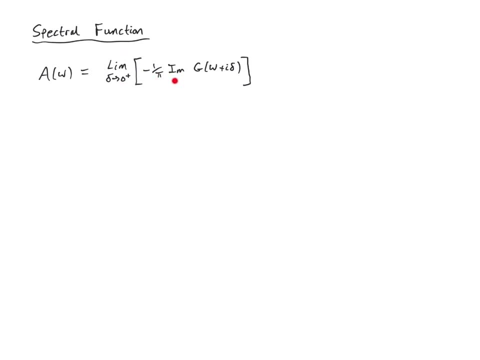 of delta goes to 0 plus of minus 1. upon pi of the imaginary part of the corresponding retarded Green's function For a single quantum orbital, we derived that the retarded g of z is equal to 1 over z minus epsilon, which gives a spectral function. a of omega is simply the 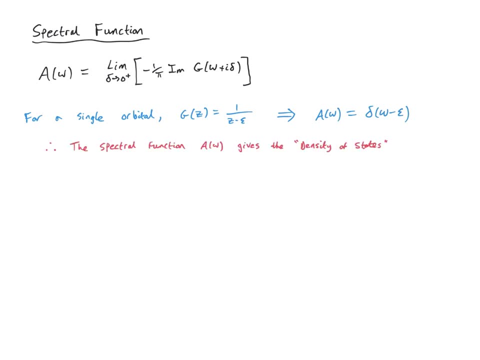 delta function, delta of omega minus epsilon. The spectral function a of omega is simply the delta. omega gives the so-called density of states. Now for the simple case that we've considered, involving a single quantum orbital, the spectral function is simply a delta function. This is a. 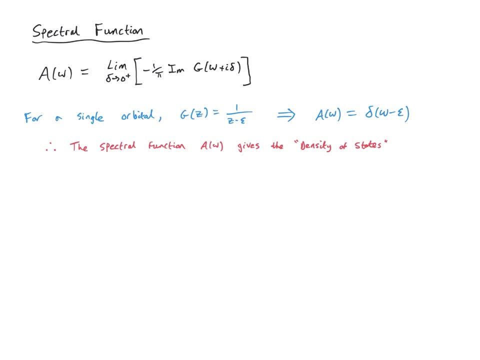 very trivial example. We have a single state in the system located at omega equals epsilon. Therefore, when we're looking at a of omega as a function of omega, we have zero until we hit omega equals epsilon and then this delta function basically counts- a single state for us, Notice. 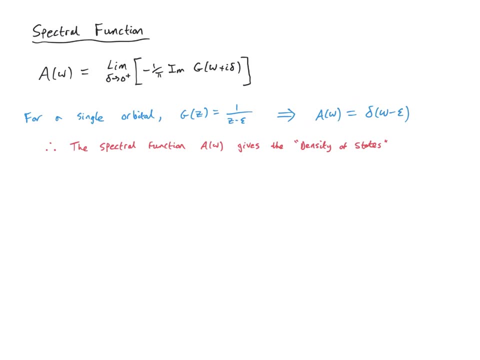 that the integral over all omega of a of omega is equal to one, The total density of states is normalized to one. The spectral function, a of omega, can therefore be thought of as being a probability distribution containing the probability of finding a state of a given energy. 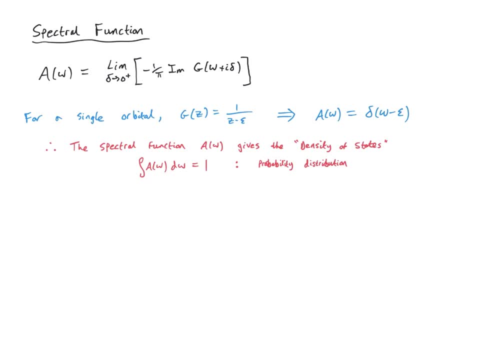 For a system of just a single orbital, we have just a delta function located at the energy of that state. We can also reconstruct the retarded Green's function with a knowledge of the spectral function a of omega. However, given that the retarded Green's function g is an analytic function of the complex variable, 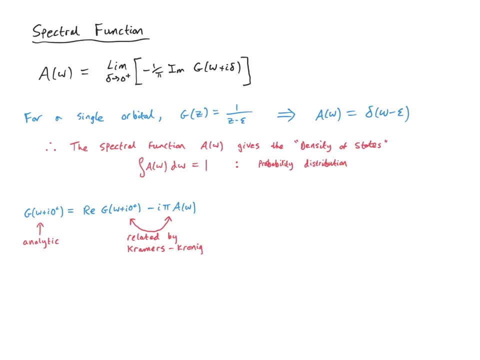 z. we know that the real and imaginary parts are related through the Kramer's cronic transformation. Recall here that an analytic function of a complex variable, z, is one that has a well-defined and convergent Taylor series in powers of z. We can use the Kramer's cronic relation to obtain the 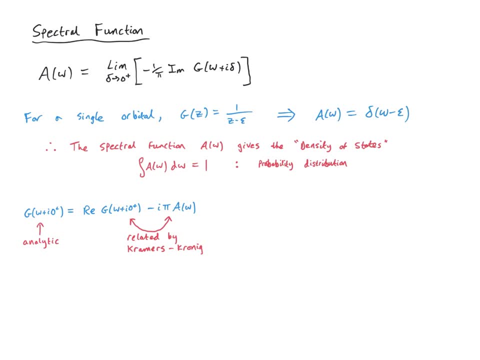 spectral representation of the retarded Green's function g of z for any complex z. We can therefore write g retarded in this fashion, purely in terms of the spectral function. As for the real part of g, we can evaluate it simply as one over omega minus epsilon, provided that omega is not equal to. 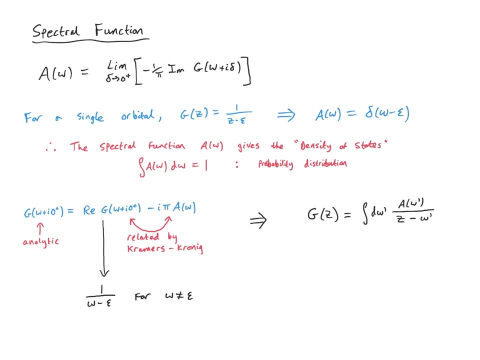 epsilon. This is referred to as the principal value of one over z minus epsilon. In this case, the real part of g looks something like this: and this is the integral function For the real part of g. we can take this function and derive the: 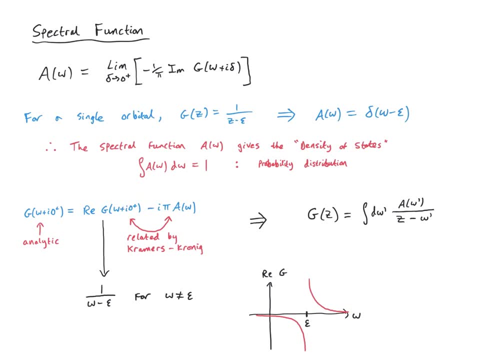 integral function of the new qui- ket G drawn here. The integral function g is the integral function of the real divergence around epsilon. The infinitesimal imaginary part of the frequency omega plus i0 plus here regularises this function. so there is no real divergence at omega equals epsilon. But for all intents and purposes, when we 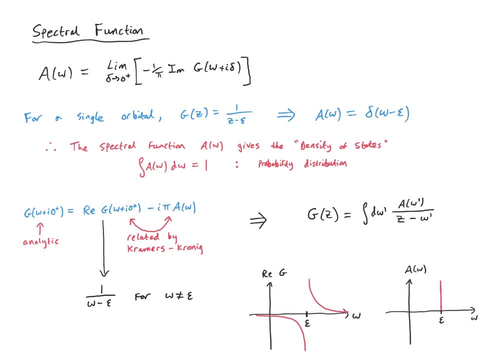 are not at omega equals epsilon. we simply see a regular function, one over omega minus epsilon. rather an interesting one. The imaginary part is only finite when omega is equal to epsilon, when we get a delta function, whereas the real part is only finite and regular when omega is. 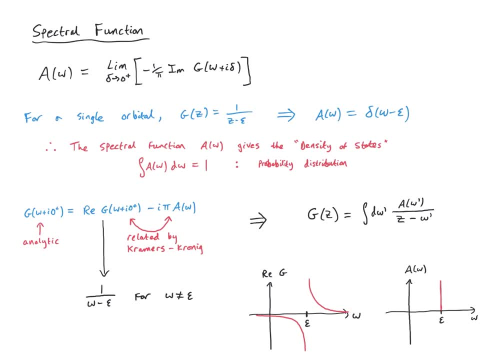 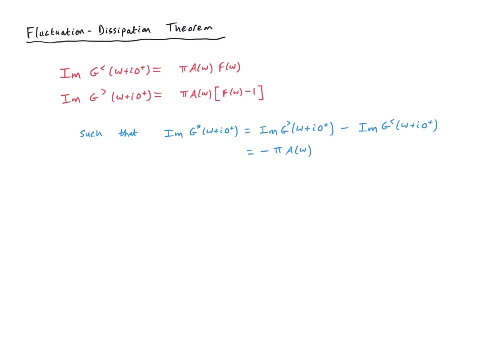 not equal to epsilon, in which case we get 1 over omega minus epsilon. From our explicit expressions for the g lesser and g greater obtained by the Laplace transformation of a complex variable z, and then sending the imaginary part to a positive infinitesimal, we can relate the lesser and greater. 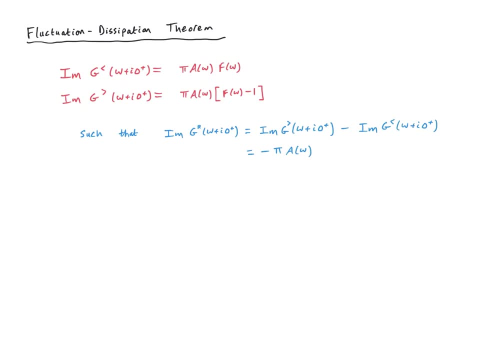 Green's functions to the spectral function a of omega on the right hand side. Indeed, given that g retarded can be expressed as g greater minus g lesser, I can take the imaginary part of both sides of the equation and simply relate the imaginary part of g retarded. 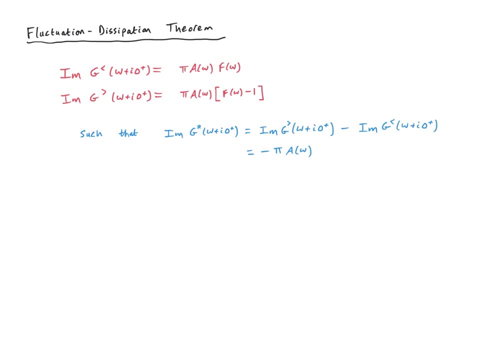 to the spectral function And of course we recover the definition of the spectral function that minus 1 upon pi of g retarded is a of omega. Previously I mentioned that it was not so simple to relate g retarded as a function of pure real frequency omega. 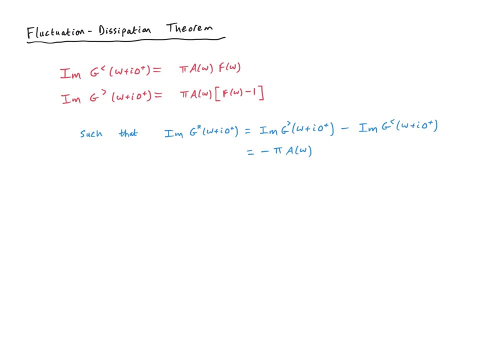 obtained by the regular Fourier transformation in terms of the Fourier transforms of g greater and g lesser. However, the spectral function provides a means to connect these objects, The Fourier transform to real frequency. omega of g lesser of omega and g greater than omega can now be cast in terms of the spectral 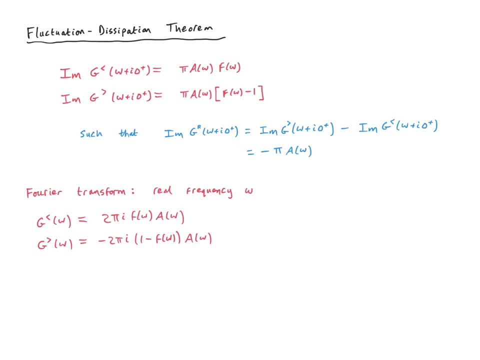 function a of omega. We've derived this explicitly here because g lesser of omega and g greater of omega were expressed in terms of the delta function, omega minus epsilon for a site of energy epsilon, and we also related the spectral function a of omega to the delta function. However, it turns out that these 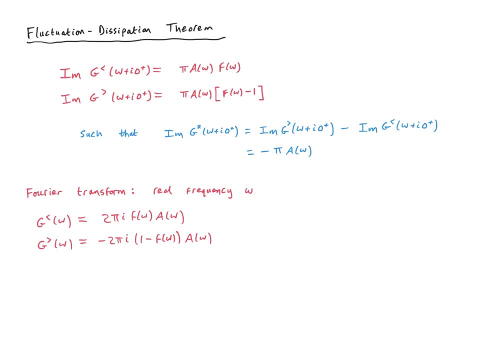 expressions are totally general and apply in all cases. We can prove that by the so-called Lehmann representation, which we'll talk about in a future lecture. These important relations are known as the fluctuation dissipation theorem. They relate the occupations of a site to the spectral functions. 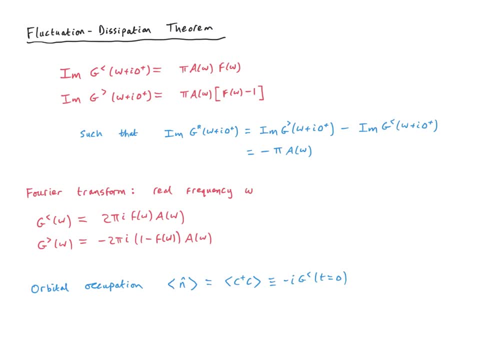 We can see this by writing the orbital occupation, which is the expectation value of the operator n hat, which can also be written, of course, as the thermal expectation value of c, dagger c. in terms of our lesser greens function, We can write it as minus i g lesser evaluated at t equals zero. This is then. 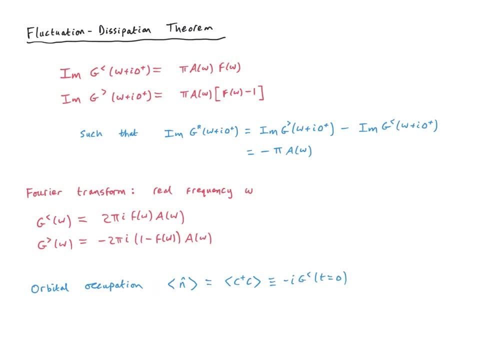 the equal times lesser greens function which gives us the orbital occupation. We can obtain g lesser of t from g lesser of omega using the inverse Fourier transform. We write one upon two pi times integral d-omega of e to the minus i omega t times g lesser of omega. 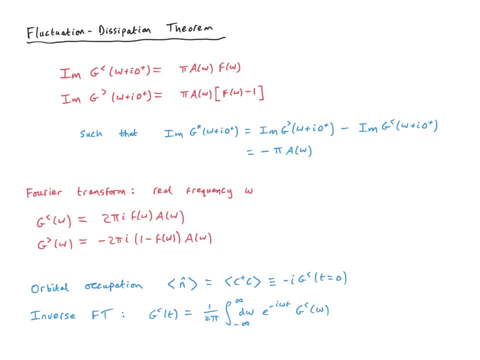 The zero time lesser greens function is therefore simply obtained by setting t equals to zero on the right-hand side, which then just means that we'd be able that we integrate g lesser of omega over all omega. We can express the orbital occupation which is the expectation value of n hat then simply as minus i upon 2 pi, integral d omega. 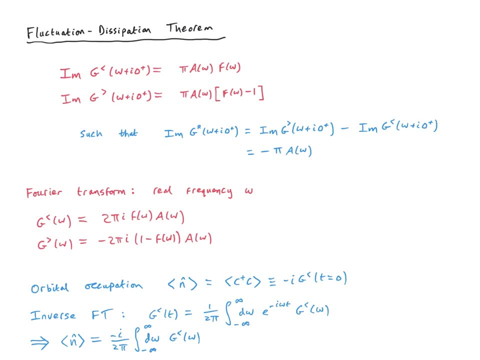 of g lesser of omega. Substituting our expression for g lesser of omega into this integral, in terms of our spectral function, then gives us the following: The orbital occupation is given as the integral d omega of the Fermi function. f of omega times the spectral function a of omega. 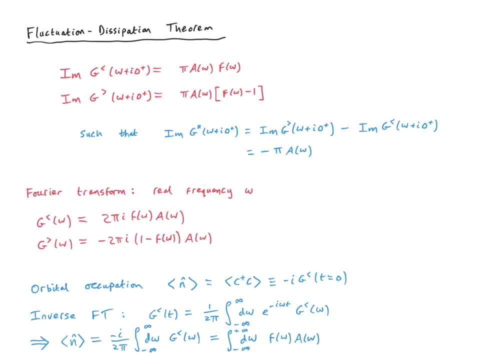 and this is an important result. It tells us how the orbital occupation is related to the spectral function. The orbital occupation is something that depends on temperature. of course, The spectral function does not depend on temperature, but we see how temperature enters this equation through the Fermi functions. Just a final comment on this, This formulation. 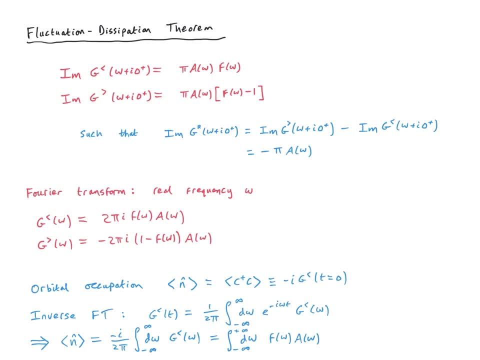 involves Green's functions of the real frequency omega, and we were able to do the inverse Fourier transformation here. Of course, we could have used these equations at the top in terms of our complex variable z, but then we would have had to have done the inverse Laplace transformation, which is a bit 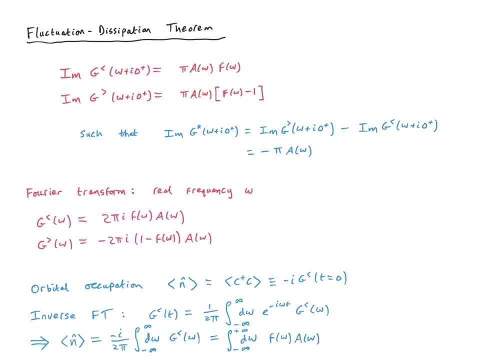 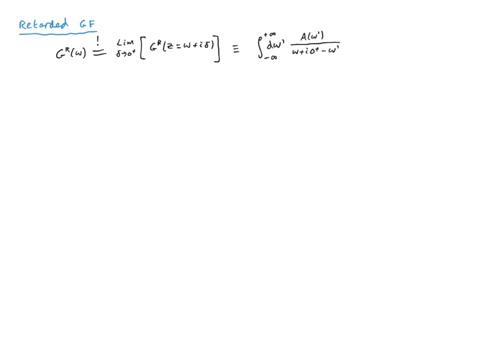 more cumbersome. Of course, they both give the same answer, but this version involving the inverse Fourier transformation is certainly easier. Finally, we're in a position to show that the retarded Green's function as a function of the real frequency omega, as would be obtained by a regular Fourier transform, can be expressed: 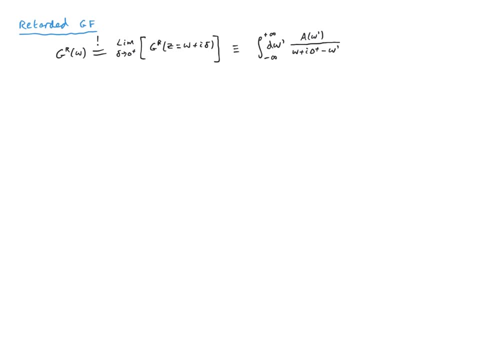 in terms of the retarded Green's function as a function of the complex variable z, as we take the imaginary part to be a positive infinitesimal. We can also express this in terms of the spectral representation in the following way: There are another class of 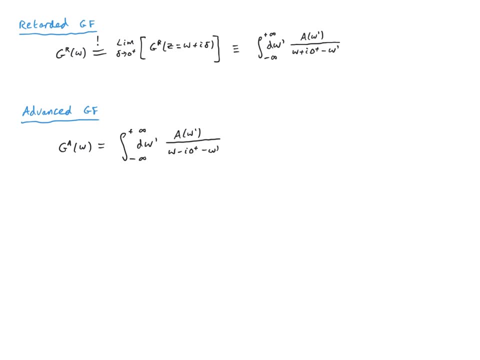 Green's functions that I've not yet mentioned, called the advanced Green's functions, contrary to the retarded Green's functions, However, the only difference in the definition is that on the bottom here we have omega minus I0+ rather than omega plus I0+ for the retarded Green's function, And therefore, since the 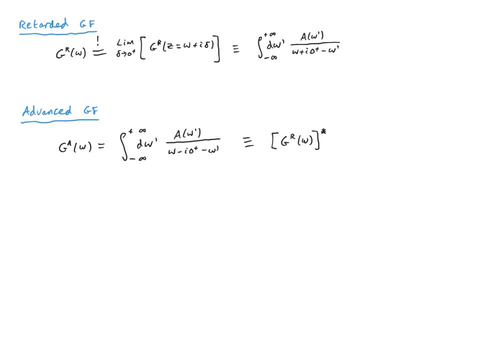 only difference is the sign of the imaginary part. we can obtain g advanced simply by taking the complex conjugate of g retarded, and this is really the only difference. Sometimes you'll see these advanced Green's functions mentioned in books or papers. However, we won't discuss. 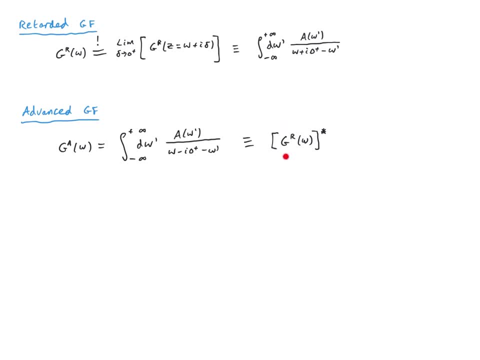 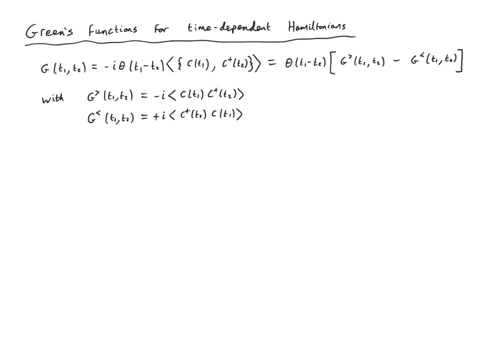 them further in this course. We'll just focus on the retarded Green's functions and suffice it to say that if we wanted the advanced functions, we can obtain them simply by this relation. Now I want to do an example of a situation with a time-dependent Hamiltonian In that 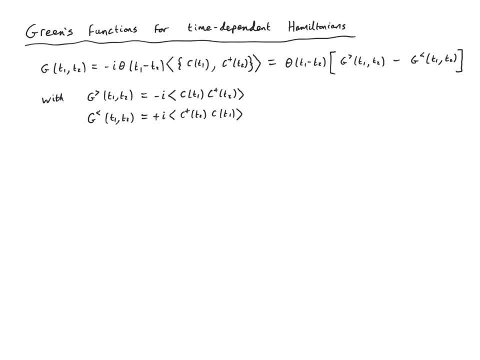 case we have Green's functions that depend explicitly on two time variables. Here I've written the retarded Green's function in terms of its original definition, and one can of course express this in terms of the greater and lesser functions. These greater and lesser functions are written down here for the case where we have t1 and 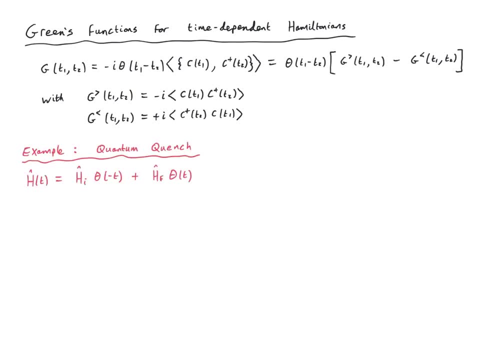 t2 being arbitrary times. So the example that I want to look at is a so-called quantum quench. This is a paradigmatic situation where the total Hamiltonian h on the left here has an explicit time-dependence. It is, however, a simple example of time-dependence because 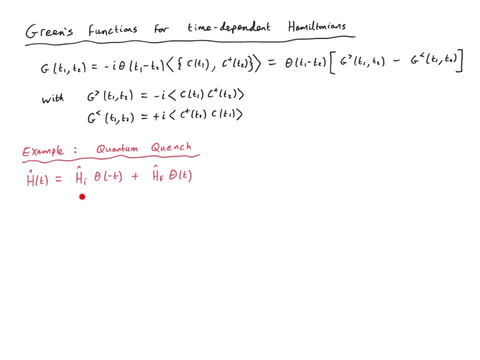 we go from an initial Hamiltonian, which is some static, time-independent Hamiltonian h, to some final static Hamiltonian h, And then we see these theta functions of minus t and theta of t here. So basically this says the Hamiltonian h is equal to. 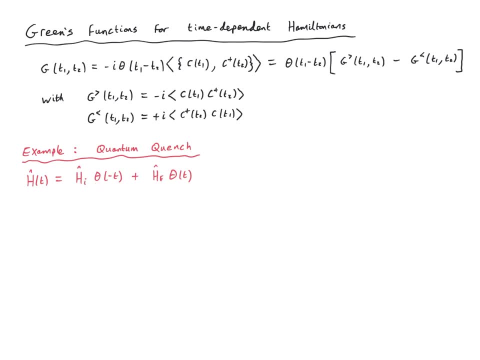 h when time is less than zero, and then it instantaneously changes to h for t greater than zero. So it's t equals zero. we just change from the initial Hamiltonian to the final Hamiltonian, And that's referred to as a quench. 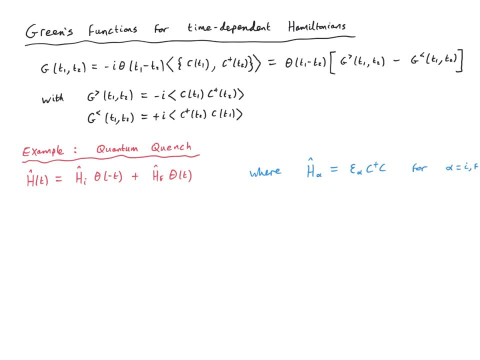 Here we'll consider the simplest possible example of this quantum quench, where our initial or final Hamiltonian- this is h, hat alpha, where alpha is either i or f for initial or final is a single quantum orbital c, dagger c, with a level energy epsilon that changes. 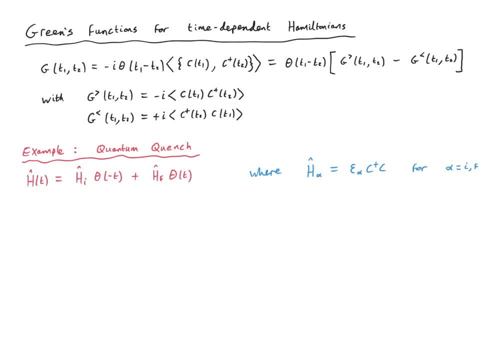 depending on whether or not we're in the initial or final state. One can think about this as having a Hamiltonian h of t that has a quantum quench, and then we have a Hamiltonian h of t that has an energy level. epsilon of t. that depends explicitly. 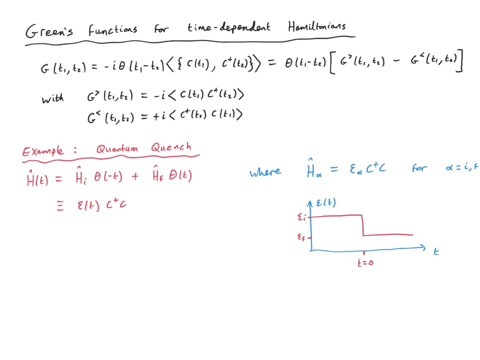 on time, and this is multiplied by the number. operator for our site. If I were to plot epsilon of t as a function of time, we would see that it takes a constant value, epsilon i for t less than zero, and then discontinuously changes to epsilon f for times t greater than. 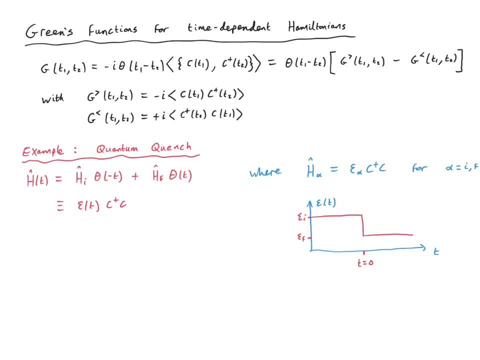 zero. So this is a very simple example of time dependence of the Hamiltonian, but we'll still see that it has some interesting physics And we can explore that physics using these time-dependent Green's functions. I should note here that for time t less than zero we have an equilibrium situation. The 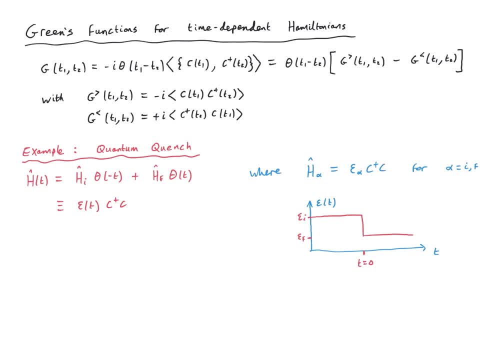 Hamiltonian is constant. If we go to the infinitely distant future, t goes to plus infinity. then we'll also have an equilibrium situation where we've relaxed to our new equilibrium with a different epsilon. this is the epsilon f. However, for finite t greater than zero, 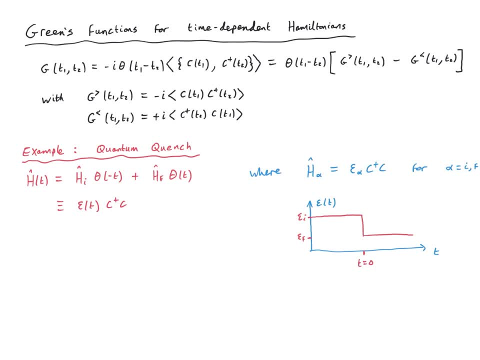 we'll see some transient dynamics when a system is relaxing from its old equilibrium to its new equilibrium, And it's this transient behaviour that we'd like to understand here. We will see that it's a little more complicated when we discuss the Green's functions of two. 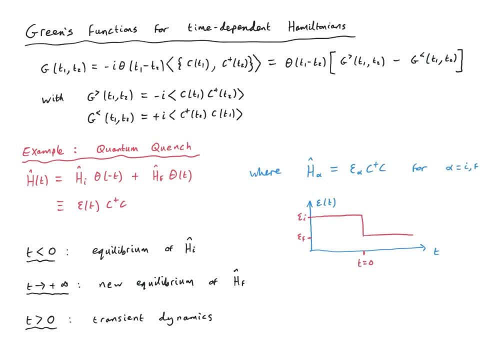 time variables t1 and t2, however, because t1 might be before the quench at t less than zero, and t2 might be after the quench at t, greater than zero, Or we could have both t1 and t2 linear. 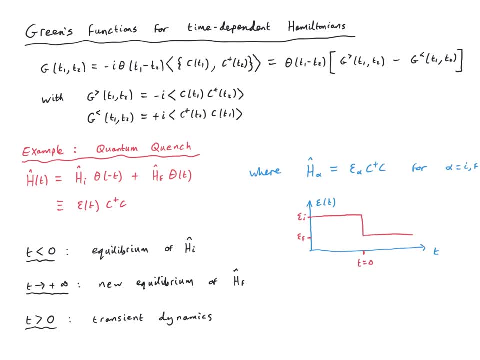 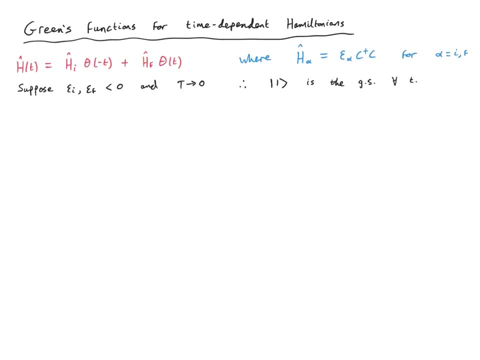 So let's just do the calculation and see what we get. So let's now suppose that the initial level energy epsilon i and the final energy epsilon f are both less than zero. This will mean that the occupied state is the ground state of the system at all times t less than zero as well as t greater than zero. For simplicity. 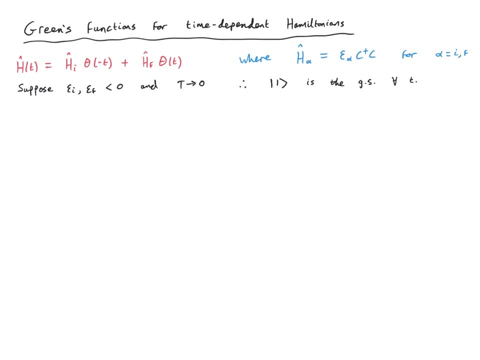 let's also specialise now to the zero temperature limit. This means that we'll only have excitations from this unique ground state. This immediately implies that the g greater function is actually equal to zero for all times. That's because on the right hand side here I have a C dagger. 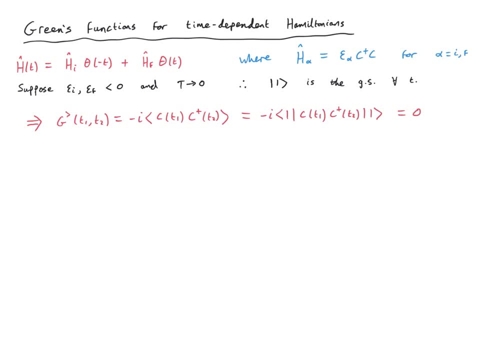 operator. But if we're only considering excitations from the occupied ground state in the zero temperature limit, then we will not be able to apply this C dagger operator. Acting with the C dagger operator at any time on this occupied state will annihilate that state. 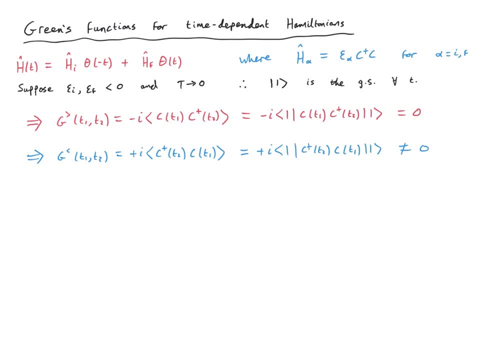 By contrast, if we look at the g lesser function, then the order of the operators is reversed. This means that here, on the right hand side, I have the annihilation operator acting on the occupied state, and this will be finite. Expressing the time-dependent operators in: 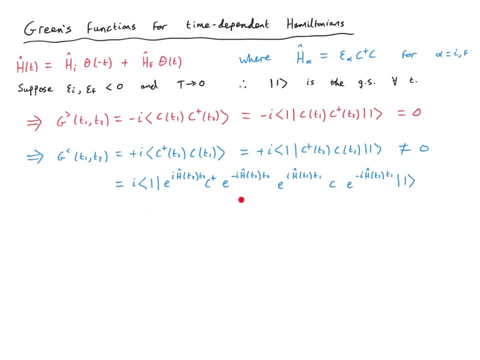 the Heisenberg form. I can now write the lesser-greens function in this way- Here I'm time-evolving the operators using e to the iht and e to the minus iht. However, the Hamiltonian has to be evaluated at the particular time of interest. For example, in this term we originally 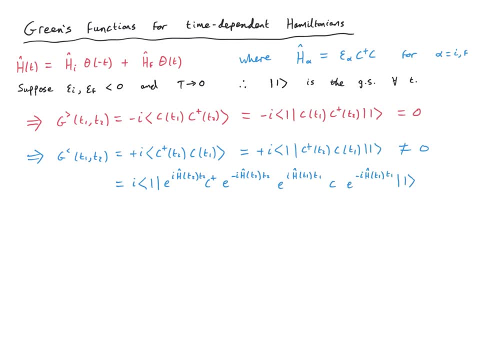 had c of time t1, and therefore we need to evaluate the Hamiltonian at that time, t1. As I mentioned earlier. we therefore need to break this down into the different regimes. First let's look at the case where both t1 and t2 are negative, In this case, h of. 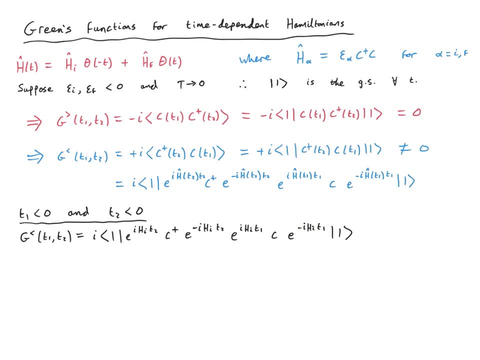 t is always the initial Hamiltonian h i, as I've written here inexplicably. now We can evaluate this string of operators as before and we simply obtain i e to the epsilon i into t2 minus t1.. We see in this case that g lesser is actually a function only of t2. 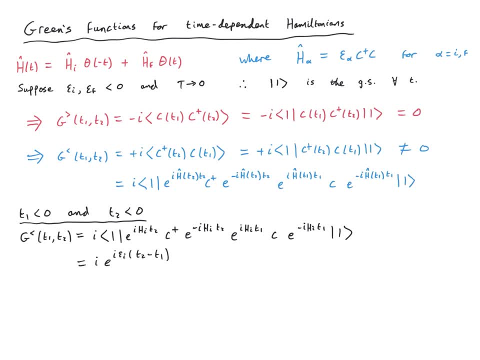 minus t1, the relative difference between t1 and t2.. This is the situation we saw previously for the time-independent greens functions. The reason why we're getting that again here is that both t1 and t2 are negative and therefore the dynamics of the system is evolving under the static, time-independent Hamiltonian h. 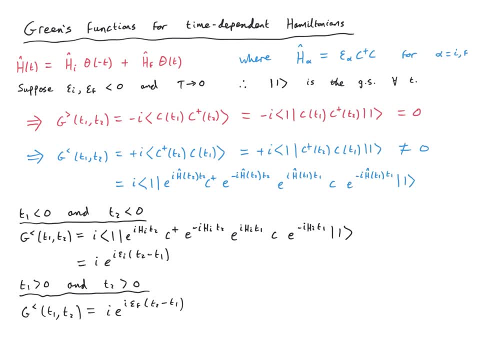 i. Exactly the same logic holds when both t1 and t2 are greater than zero. Here the system is evolving under the final Hamiltonian h f, which is time independent. The greens therefore look exactly the same, except we simply replaced epsilon i with epsilon f. 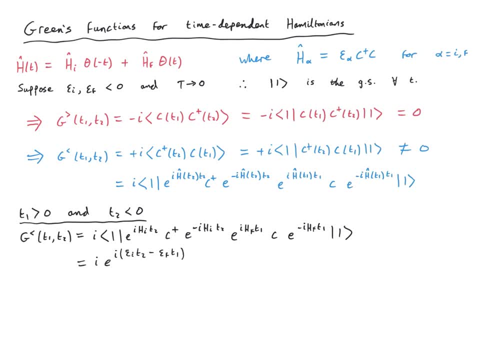 The more interesting case arises when t1 and t2 have different signs. For example, let's look at the case when t1 is greater than zero, that's after the quench, and t2 is less than zero before the quench. Therefore, in the string of operators, this first term, which is evolved at 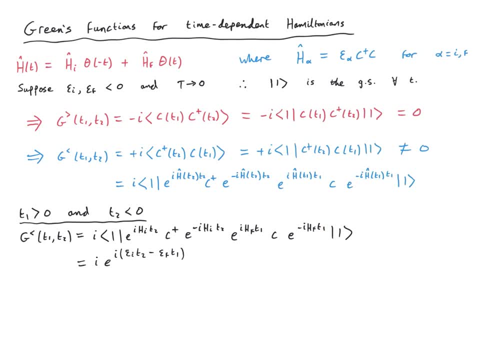 time t1, applies to the final Hamiltonian hf, whereas this operator is evolved under the initial Hamiltonian because we're at time t2, which is less than zero. When we evaluate this, we find that g lesser is i e to the i, epsilon i, t2 minus epsilon f t1.. So let's now discuss the Laplace. 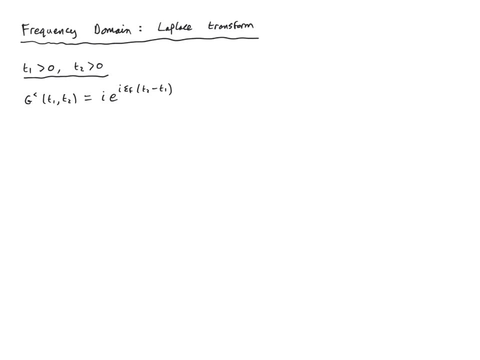 transformation to the frequency domain of these Green's functions. First of all, we have to take care of the fact that we have two time arguments: t1 and t2.. We'll therefore introduce the label t to mean the average time between t1 and t2, and the label tau to indicate the time difference. 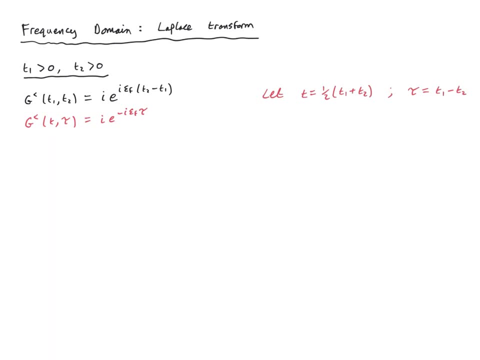 t1 minus t2.. With this change of variables I can write g lesser, as a function of t and tau is equal to i, e to the minus i, epsilon, f, tau. We now perform the Laplace transformation on the variable tau. This is the time difference. 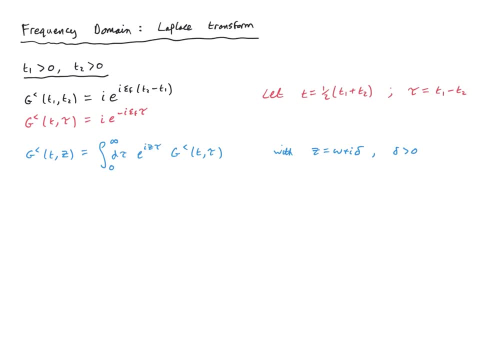 This will give us a Green's function, g lesser, which is something that depends on time, but also on this complex variable z. We want to keep this time argument here because we want to know the Green's functions as a function of the real time in the system. 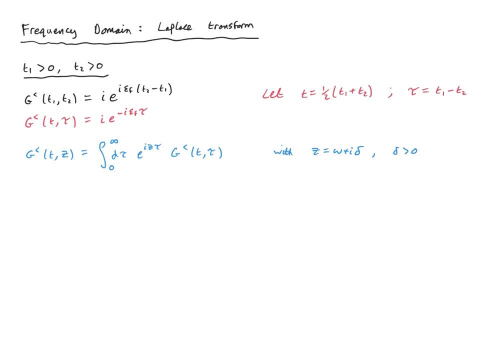 The dynamics of the system in these correlation functions are encoded in the time difference, which is tau, and this is the variable that we're Laplace transforming to the complex variable z. Evaluating this integral explicitly, we obtain minus one over z, minus epsilon f, and we see on the right-hand side: 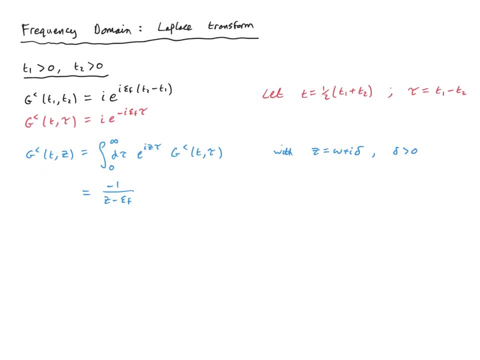 that this Green's function is not depending explicitly on the time label t. This is actually as expected because, as we argued right at the beginning, when both t1 and t2 have the same sign, we'll have an equilibrium situation, In this case, with t1 and t2 both greater than zero. 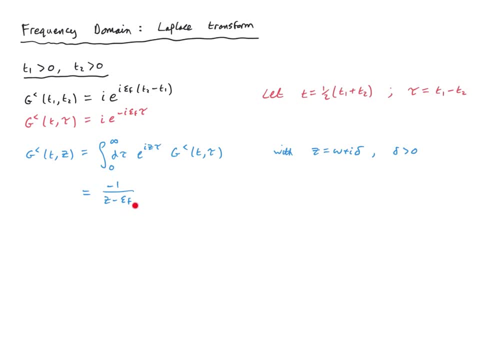 the dynamics are controlled by the final Hamiltonian and therefore we have epsilon f as here As before. we can now define a retarded Green's function of the complex variable z in terms of g greater minus g lesser. It's just that now we carry this additional time label t. 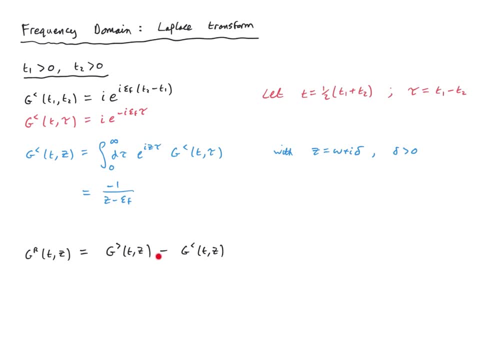 We also argued that at zero temperature this g greater function was equal to zero and therefore overall we have that the retarded Green's function is simply one over z minus epsilon f. Again, this confirms our original assumption that if both t1 and t2 are x, then we should obtain the equilibrium Green's function for the 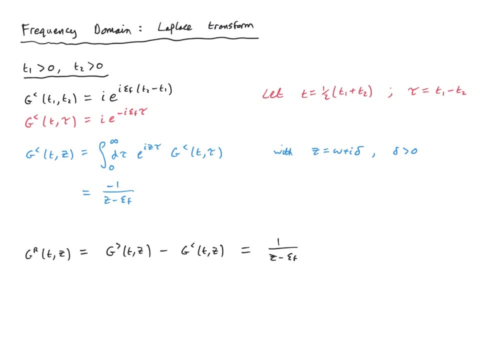 final Hamiltonian, which we know already, is one over z minus epsilon f. In an exactly analogous fashion, if t1 is less than zero and t2 is less than zero, then we have an equilibrium. Green's function for the initial Hamiltonian g lessor of t in tau takes this form: 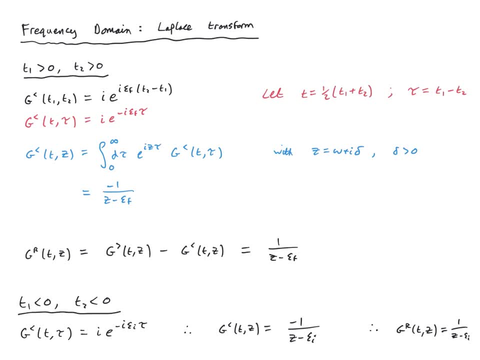 performing the Laplace transformation to the complex variable z from tau, we obtain chain g, lesser of t and z, and then finally, just as before, we can obtain the retarded Green's function. This again takes exactly the form we expected, with 1 over z minus epsilon i, now with epsilon i being the level energy for the. 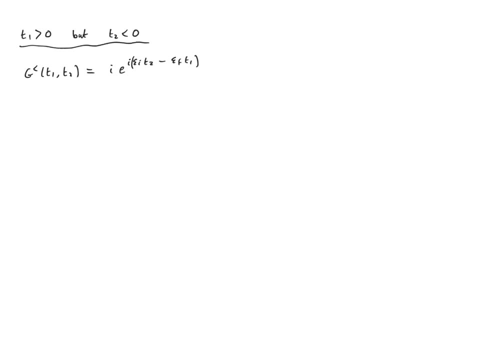 initial Hamiltonian. Much more interesting is the case when t1 is greater than 0 and t2 is less than 0, in which case we can define a lesser Green's function of our two times t1 and t2, which we worked out earlier as this: 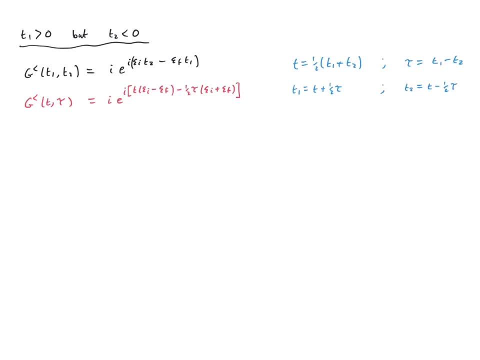 thing. Let's now convert this to t and tau. We can write g lesser of t and tau as i e to the i t, into the difference between epsilon i and epsilon f, minus a half tau of the sum of epsilon i plus epsilon f When we perform the Laplace. 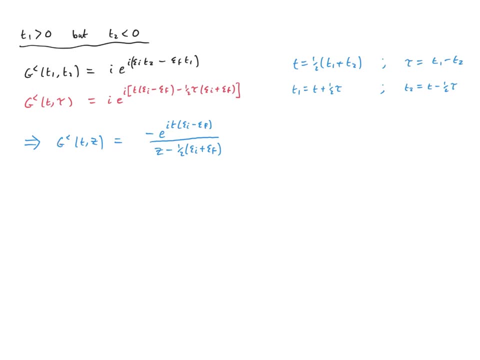 transformation of this, we obtain g lesser of t and z in the following form: The specific function a of t and omega therefore takes this rather unusual form. We see that we have a delta function exactly at the average position of epsilon i and epsilon f, but that the amplitude of this has this oscillatory form in time. 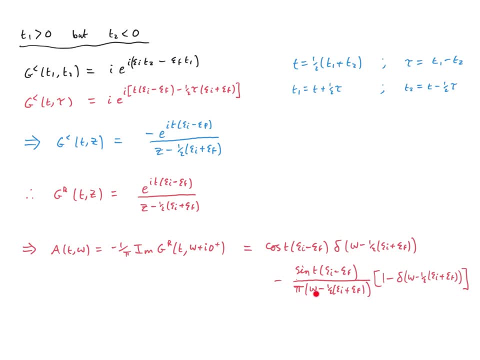 Then we also get this piece corresponding to the real part of the retarded Green's function times, the sine of t, epsilon i minus epsilon f, and this is finite whenever we're not exactly at the pole position, omega equal to t. So the formula for this is not a feature of equilibrium, but it's something that 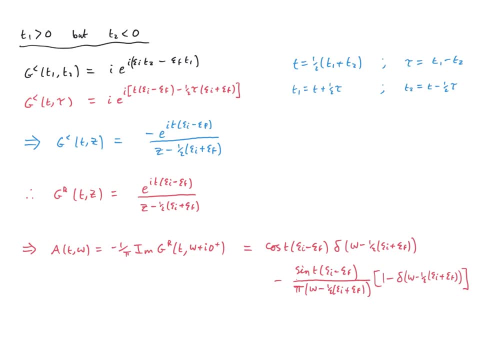 can happen out of equilibrium due to these quantum quenches. You'll also notice that this spectral function actually can be negative. This is not a feature of equilibrium spectral functions, but it's something that can happen out of equilibrium due to these quantum quenches. 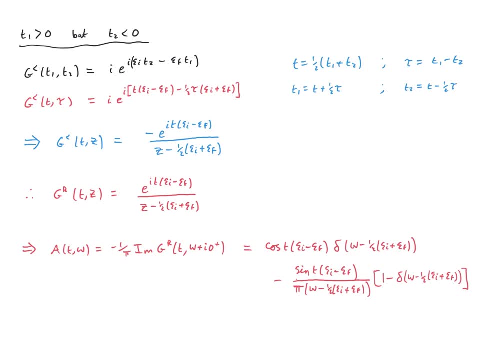 So this was a simple example of a time-dependent Hamiltonian and time-dependent Green's functions that arise for such systems. In this particular case we considered the zero-temperature quantum quench case, which is one of the simplest. It quickly gets more. 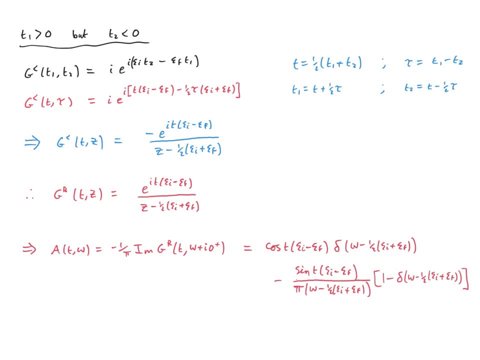 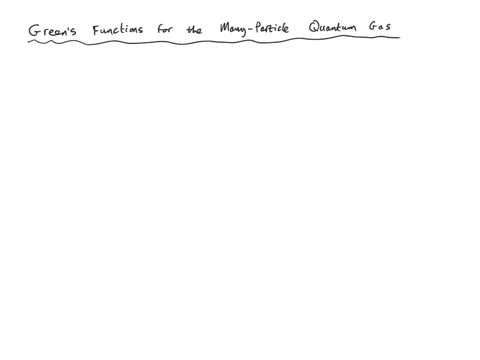 complicated because in this case we're looking to find out the love of time, as opposed to with more complicated systems, but the basic ideas are the same. The final topic of today's lecture is how we calculate Green's functions for many particle systems. This is actually a big topic. 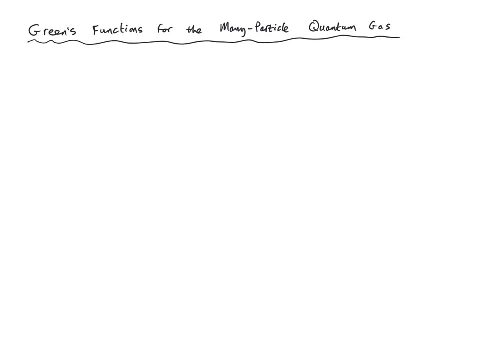 that will be developed further in the future lectures. however, today I just want to touch on a simple example of the quantum gas. So far we just considered a single quantum orbital. in fact, now we're going to go back to the time independent case, but we're going to add more. 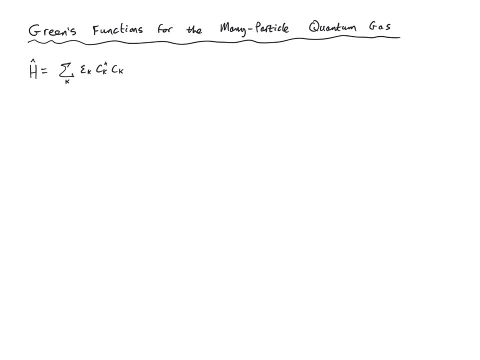 orbitals. A quantum gas is one that is written in this so-called diagonal representation. We have a bunch of quantum orbitals, but they don't talk to each other and all of the electrons in this system are independent. This is a quadratic Hamiltonian, meaning that we just have pairs of these fermionic 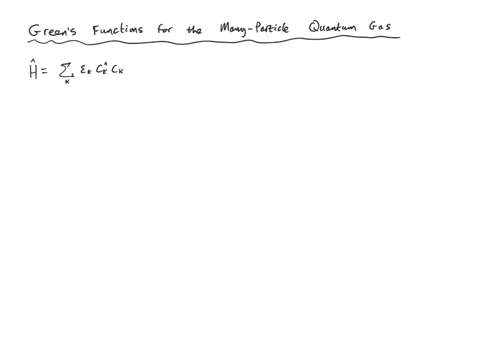 operators, and there are no electronic interactions in the system. Furthermore, each of these orbitals is decoupled from all of the others. The important simplification in the case of a quantum gas is that the exact many particle eigenstates of this Hamiltonian are product. 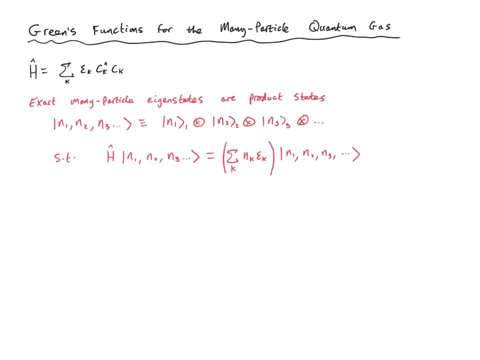 states in the occupation basis of each orbital. We can write an exact eigenstate of the system in this ket notation involving the orbital occupation for site number one, two, three and so on, and we can express this simply as the direct product of these complex vector. 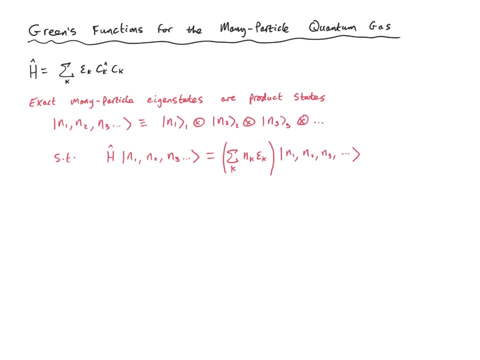 spaces for orbital one, orbital two, orbital three and so on, where n1, n2 and n3 are the occupation numbers. This is an exact eigenstate of the Hamiltonian, because if we apply h-hat to this ket, we get the ket back again multiplied by some scalar quantity, that's the energy, in this case of. 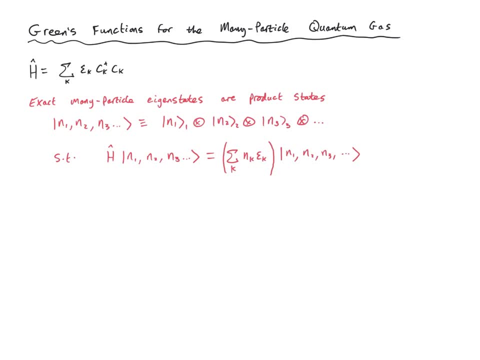 course, which is simply the sum over the orbital occupation for a given site times the site energy, and we sum over all sites. These nk's being summed over here are not operators. they're simply the quantum numbers corresponding to the orbital occupation in this ket. So let's now have a look at the corresponding Green's functions for this system. I can define: 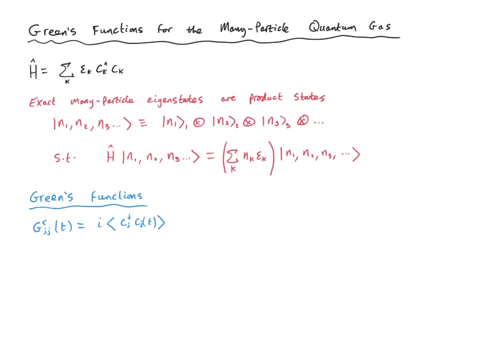 a lesser Green's function, for example for orbital number j. I will label this g-lesser with the subscripts j, j. Since the Hamiltonian is time independent, I know that this will be a Green's function of a single time variable, t. I express this as i times the thermal expectation. 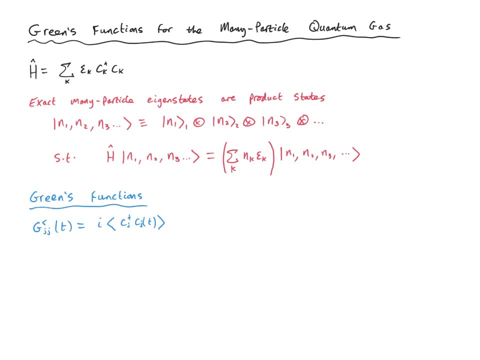 value of the operator cj dagger multiplied by cj evaluated at time t. This is an exact eigenstate of the Hamiltonian. I can define this as i times. the thermal expectation value of the operator cj dagger multiplied by cj evaluated at time t. This is an exact eigenstate. 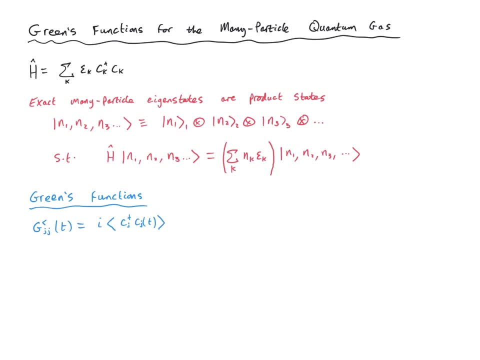 of the th And j here labels the orbital. This is therefore the local Green's function for orbital j, Using the usual definition of the thermal expectation value in terms of statistical mechanics and also the Heisenberg representation of the operator evolved forwards in time to 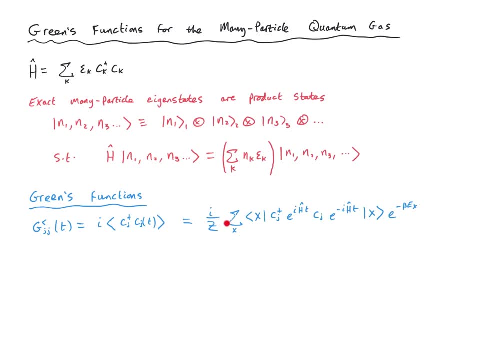 a time t, we obtain the following: Z, here is, as usual, the full partition function. these ket x's here are exact eigenstates which are obviously going to be of this product state form that I wrote out earlier. Ex is the eigenenergy, which is this object, and inside here we have this bunch of operators. 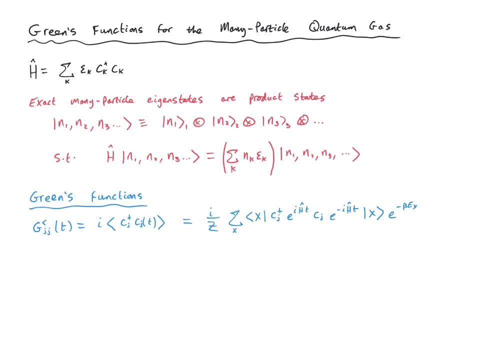 We have the creation and annihilation operators for site j, but we also also have these time evolution operators. Note here that we're summing over all possible eigenstates of our many-particle system. The important point, however, is that this cj operator and this cj dagger operator. 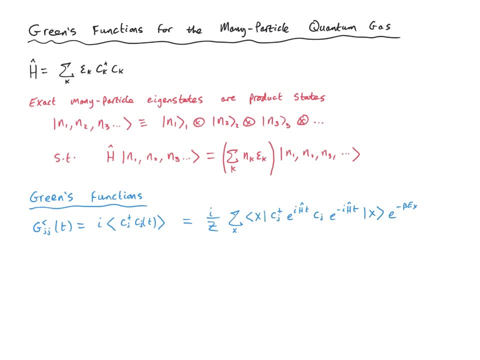 only act on site j and they commute with operators for all the other orbitals in the system. That means that, even though the eigenstate denoted ket x here involves all of the orbitals 1,, 2,, 3, and so on, these operators only act on the j-th orbital. Indeed, given that we have a ket x here, 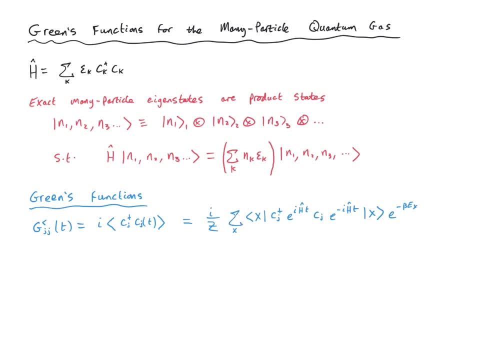 and a bra x here. these operators only act on the j-th orbital. On this side, the only thing that's changing by this string of operators is what's happening on the j-th orbital. Everything else remains unchanged Because of the product state structure of the eigenstates. one can then simply show: 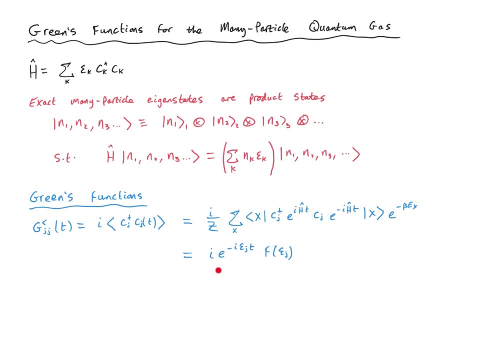 that the lesser Green's function for orbital j is equal to i e to the minus i ej t times the fermi function evaluated at epsilon j. The form of this Green's function equation is exactly the same as that which we obtained for a single quantum orbital. So we see that for the quantum gas, where we have a bunch of non-interacting, 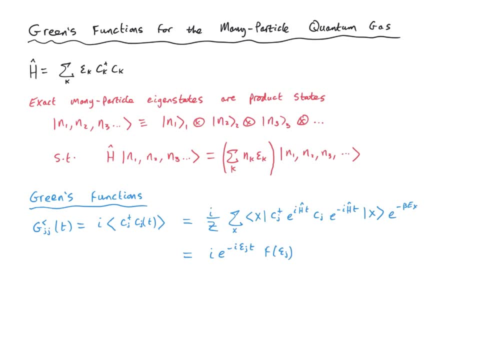 quantum orbitals that don't talk to each other. the Green's function for each of those orbitals is as if we have just a single orbital, And the same results also hold for the greater and retarded Green's functions. I will leave it as an exercise for you to confirm these results. 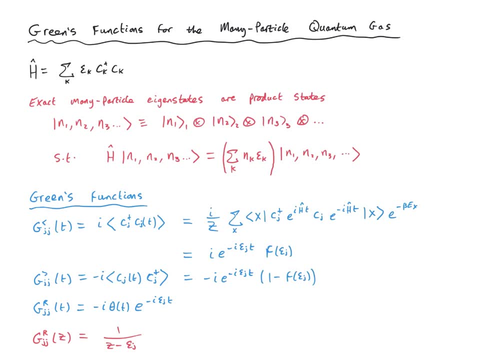 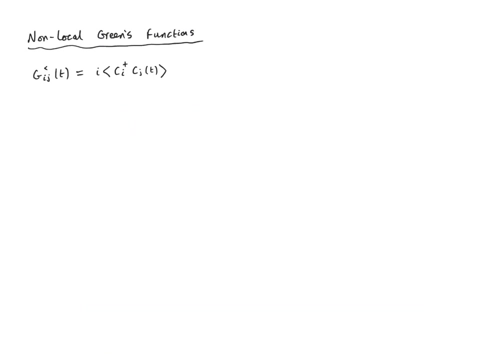 Indeed, when we perform the Laplace transformation to our complex variable z, we find that the retarded local Green's function for orbital j is simply 1 over z minus epsilon j. as you might have expected, Of course, in our many-particle system we can also define non-local Green's. 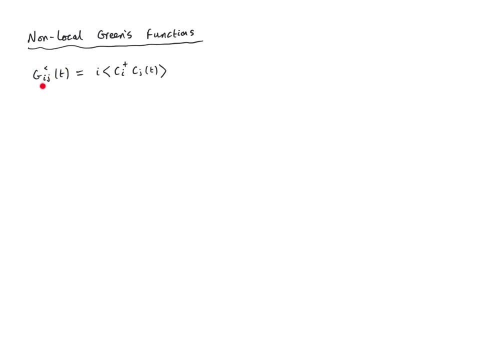 functions. For example, consider g, lesser ij of t, where i and j now refer to different orbitals. This would be defined as before. as i times the thermal expectation value of these operators, We have c dagger for orbital i and c of t for orbital j. We can write this out in the same way as before, using our definition. 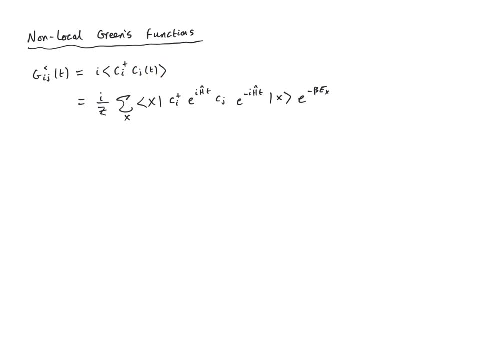 of the time, evolution of the operator and our expression for the thermal expectation value from statistical mechanics. Remember that these ket's here are the many-particle eigenstates and we're summing over all of them, all of those. We can now immediately see that this entire matrix element here is proportional. 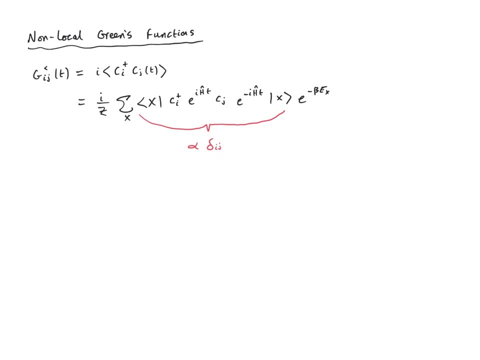 to the Kronecker delta, delta ij. That means that this object is precisely equal to zero if i and j are not the same. This can be understood by imagining the action of a cj annihilation operator for site j upon some arbitrary ket which I've labeled here in the 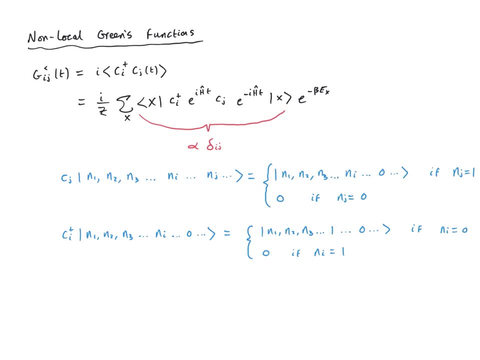 occupation basis, We see that this will give exactly zero. if nj is equal to zero, That's because we're trying to annihilate something in orbital j, and if there's nothing there, then this will give zero. On the other hand, if nj is equal to one, then I can annihilate. 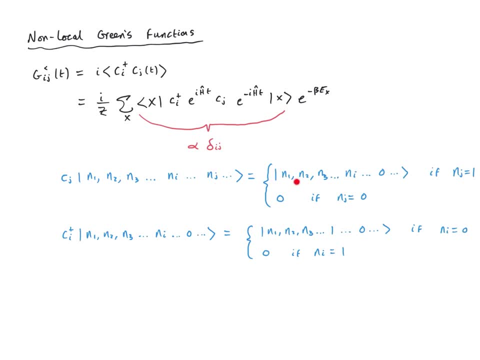 the electron in that orbital and I would obtain this ket. Let's now consider feeding this ket back in and operating on it With ci dagger, the creation operator for orbital i. this will again annihilate the ket. if ni this time is equal to one, That's because of the Pauli principle. I cannot create an electron in the i-th. 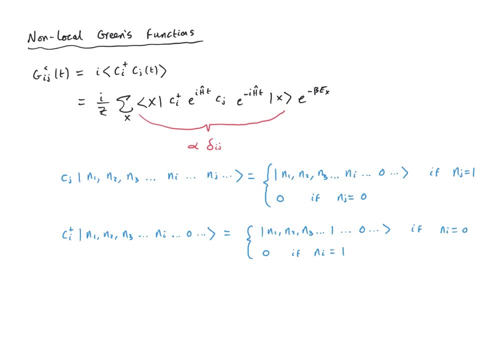 orbital if it's already occupied. On the other hand, if ni is equal to zero, then I will get this ket. So the only non-zero contribution when I act with ci, dagger, cj is a ket where there are no electrons in the i-th orbital. 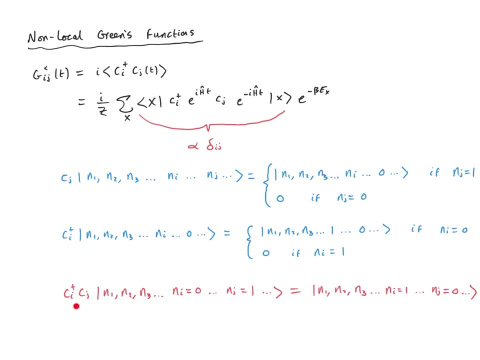 And one electron in the j-th orbital. When I act with this operator, I then end up with a state with one electron in the i-th orbital and no electrons in the j-th orbital. Note also that the occupation numbers of all of the other orbitals are exactly the same on the left-hand. 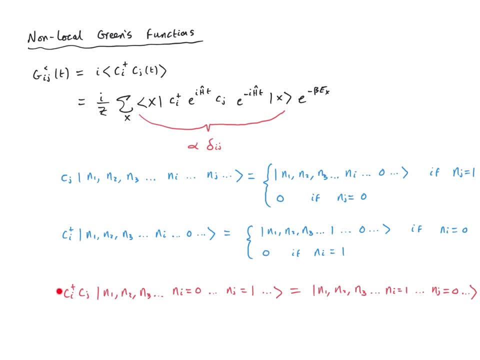 side and on the right-hand side The ci dagger, cj operator doesn't affect the number of electrons in all of the other orbitals. Now, the important thing is is that the matrix elements are going to be the same as they are in the j-th orbital. So if I want to multiply this equation by the 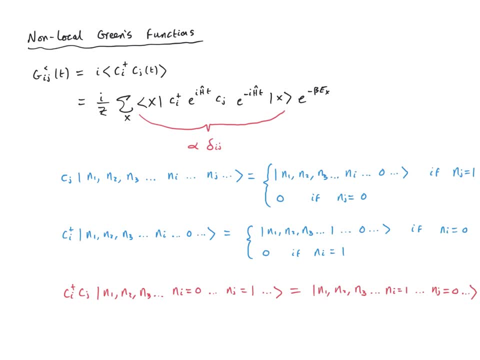 bra of this state, then I obtain this matrix element and this is equal to zero, Because on the right-hand side I would have the bracket of this state with the bra of this state and the bra of this state with the bra of this state and the bra of this state with the bra of this state. 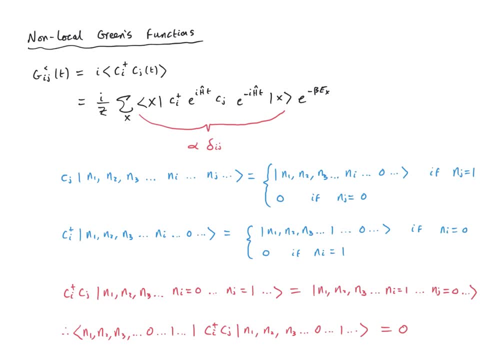 So this shows that if the operators i and j are not the same, then that means that this matrix element will be equal to zero. Fundamentally, this is because the Hamiltonian conserves the individual particle numbers of the different orbitals and this operator, ci, dagger, cj is.